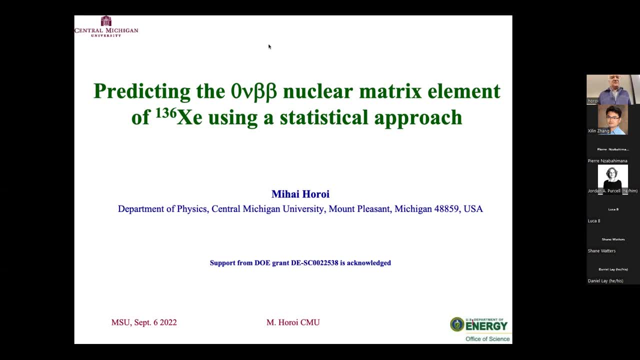 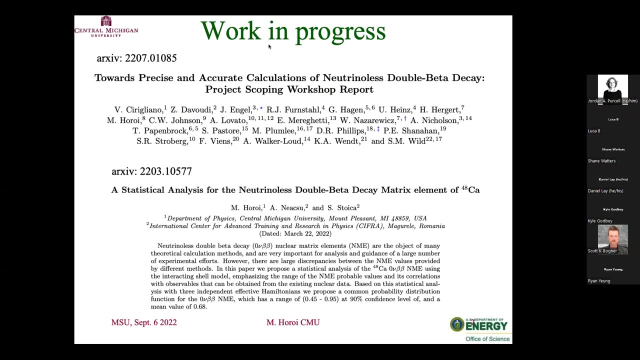 years. but more recently we were interested to kind of put some error bars on these matrix elements And I have this on my you know list for a long time but things are kind of delayed. But recently we have this workshop last February and 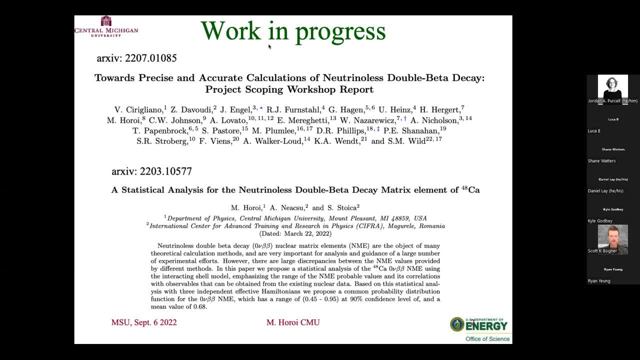 I guess some of the people which are here are organizers and participating And actually I started doing this for Calcium 48 a few months before, knowing that the workshop will come up And we have this archive paper which was submitted and we're waiting for the final. 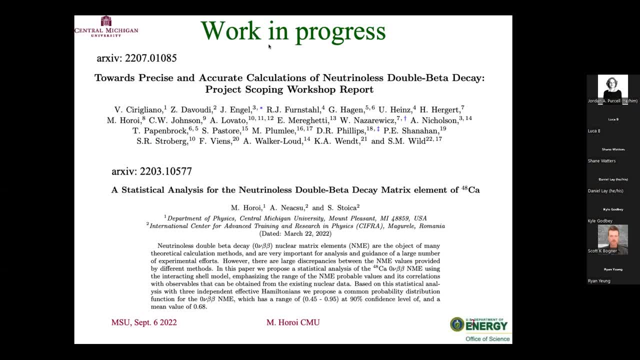 decisions. here. I'm not going to talk about Calcium 48.. Calcium 48,, of course, is a simple case because it's a little easier to calculate, It's accessible to many methods And we started with that, And I'm going to talk actually about the similar analysis. So in 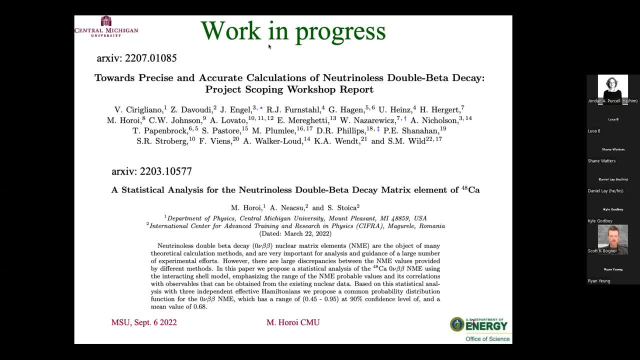 principle. you can see the prep print for the Calcium 48. So the analysis for xenon is similar, but it has some additional features. Okay, So I know that double beta decay is well known here at MSU and people would probably follow this seminar series, but I'm going to say a few words about double beta decay. 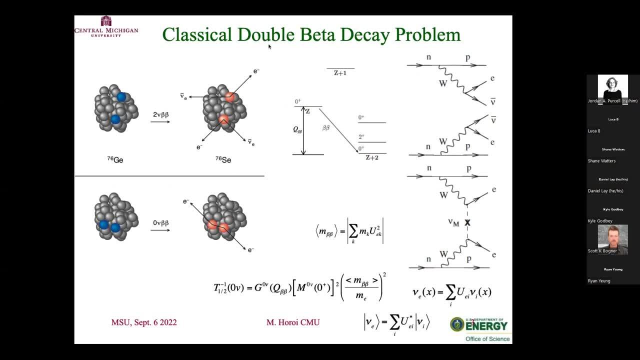 So this is a classical double beta decay problem, you know, which was kind of proposed in the 1930s: The two neutrino double beta decay which is pictured here Again. it looks like the red dot doesn't work anymore. 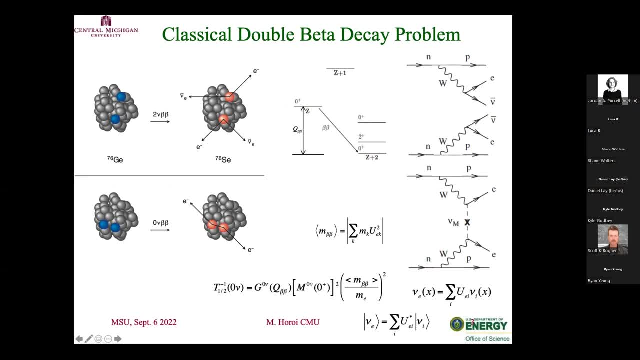 Okay, I'm going to use the arrow here. So this is a two neutrino double beta decay and it is allowed by the standard model and was measured for about 10 isotopes. And at the same time in the 1930s the neutrino less double beta decay was proposed. 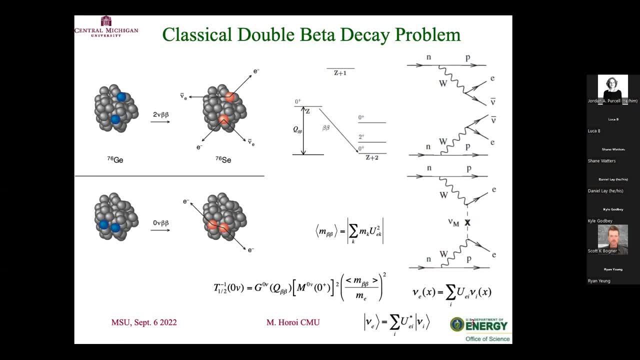 which required the neutrino to be a Majorana particle And classical scheme at the time where people thought that actually neutrino. is that better the case? more probable because there are only two particle in the final channel, so the phase space is favorable compared with two neutrino and in 1940s people start measuring uh, neutrino. 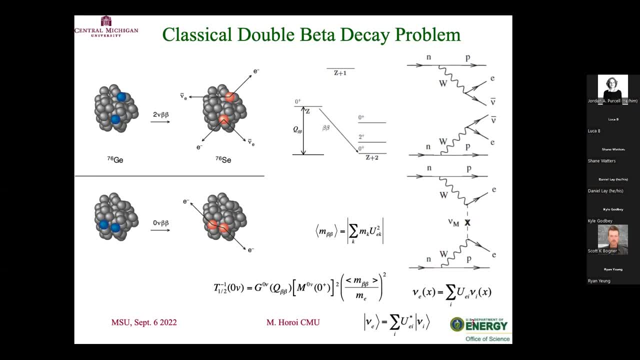 is now beta decay. they start with, i believe one of the first times it was tin-124, okay, and they didn't find anything. and i believe later on ray davis also tried to see if neutrinos are majorana and that's how the whole solar neutrino business started. but obviously in the 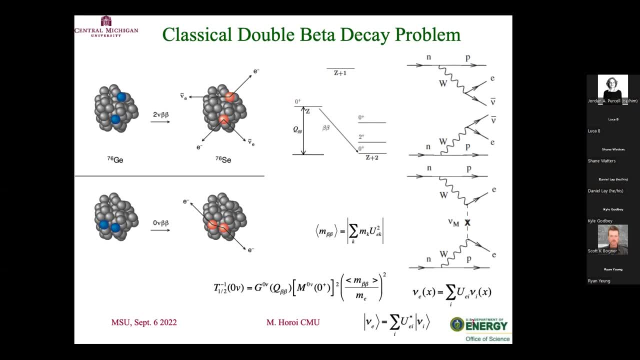 1950s, 1956-57 was a feverishly here. in physics people discover that in weak interaction the neutrinos come only left-handed. so that changed almost everything. and now the neutrinos that we get better, decay become less probable. uh, and you need to acquire mass. so in the 1930s mass was not really necessary. 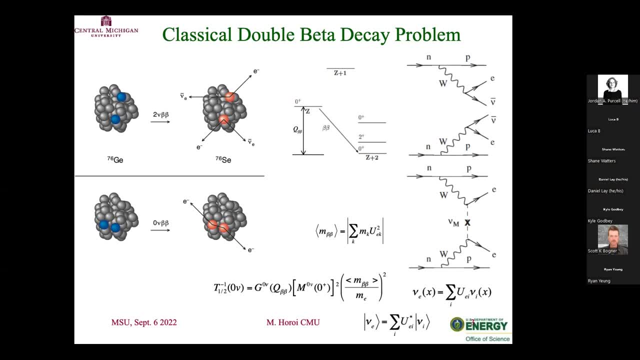 uh, but after that the mass was important and because of that for some years people are just talking about that theoretically until 2000 when, uh, neutrino oscillation experiments show that actually neutrinos have masses. okay, so that's actually, it was kind of a revival for neutrinos. 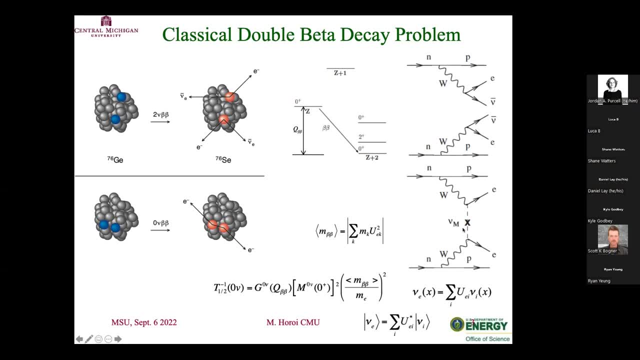 about beta decay, about this process which now is called the mass mechanism. there are many others. i'm going to maybe allude to them, but for some reason- because we already know something about this- weak interaction parameters or beyond standard model parameter m, beta, beta. we know a little bit about some of the masses and it's about the mixing angles which are in this u. 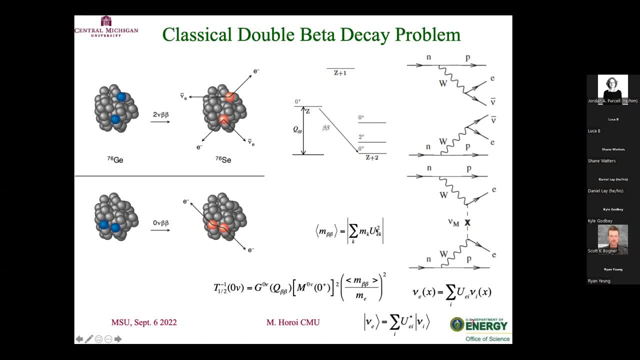 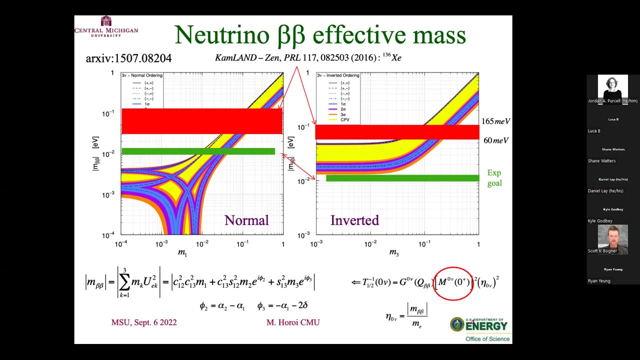 matrices. okay, so because you know a little bit about that. see, people think that, okay, we can probably find something more about that. so that's for. therefore, this picture is kind of shown in many cases, namely that because knowledge about the neutrino mass eigenstate is limited to two differences, and 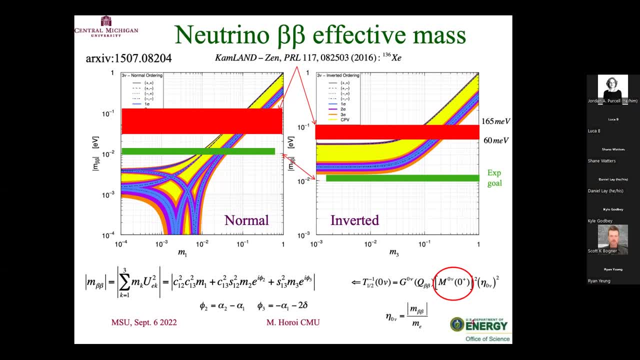 one without sign, which imply that there is a normal ordering and inverted ordering and in that case this, uh, the decay rate or reverse half-life, is proportional with some matrix element and this parameter, m, beta, beta, which is a combination of amplitudes here which are complex. 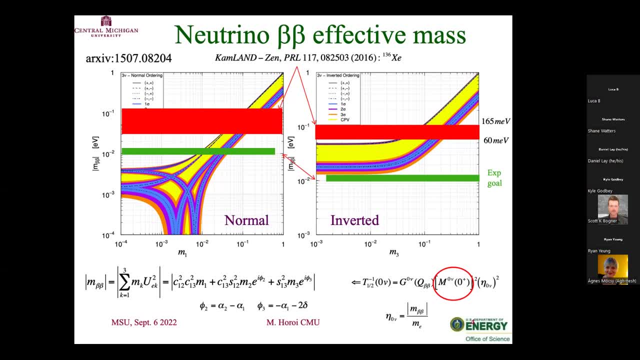 and because of that there is interference. in fact, there is interference also in the matrix element, but we can control that. so somehow, in this case, the matrix element and the uh and uh weak parameter and beta, beta is this interference and that's how we can also use this as the 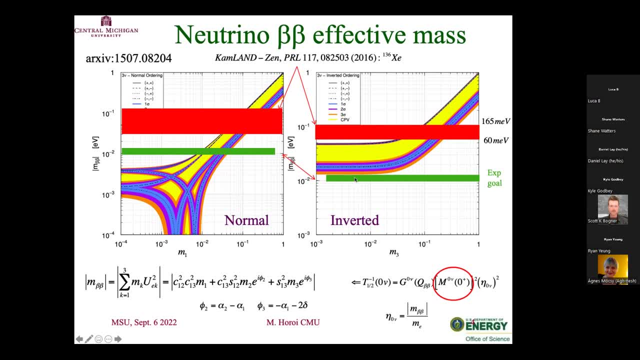 uh, comps for the everything and um, it's like a experiments are getting close, but of course it depends on the matrix element. you can see here the the m, beta, beta go between 60 mev and 160 milli electron volts based on different matrix elements, which i'm going to talk about. okay, all right, so now what? 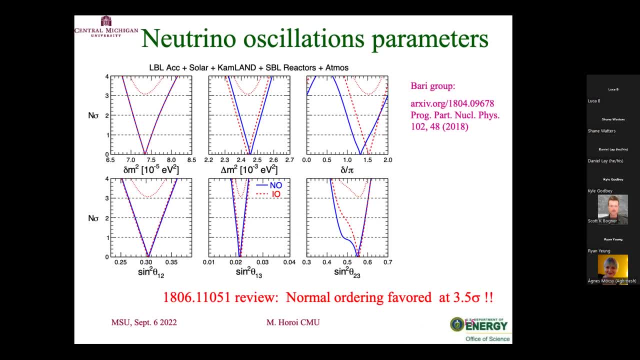 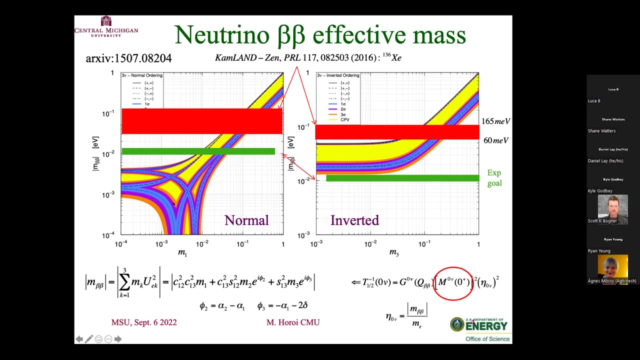 are the chances to be in one hierarchy or the other. so people are doing a lot of. there's a big business of doing a neutrino oscillation analysis and about a few years ago actually, in the inclination was towards a normal ordering. the normal ordering will actually leave open. 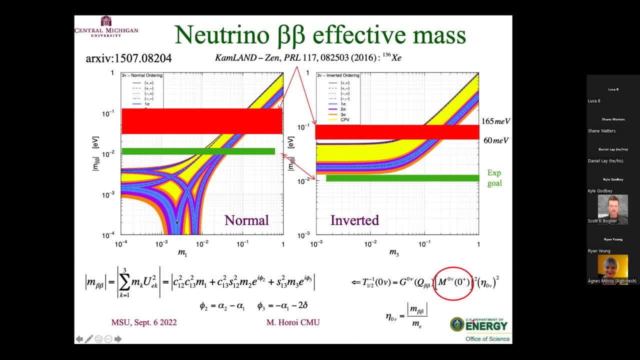 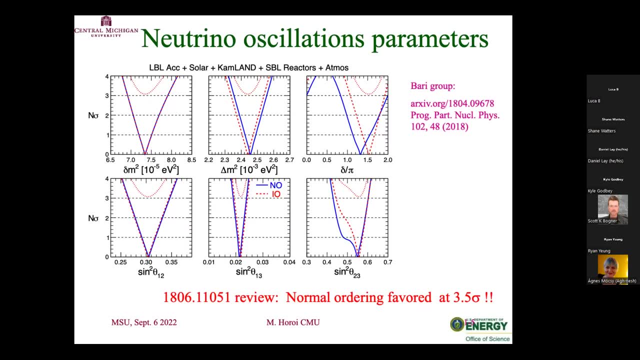 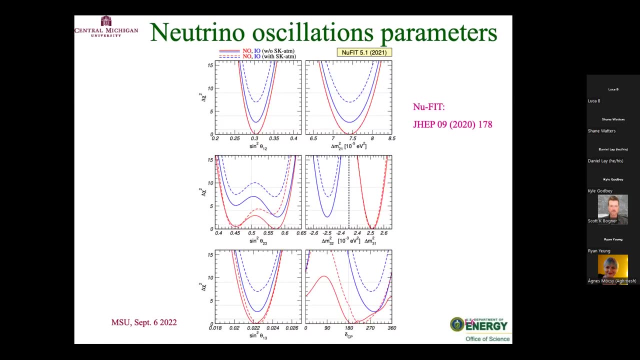 the possibility that we might not see neutrino is now better decay under this process. okay so, but apparently one of the important pieces is this atmospheric neutrino. so if you the more recently, this is the most most recent analysis at new feet. there is no really a three sigma probably. 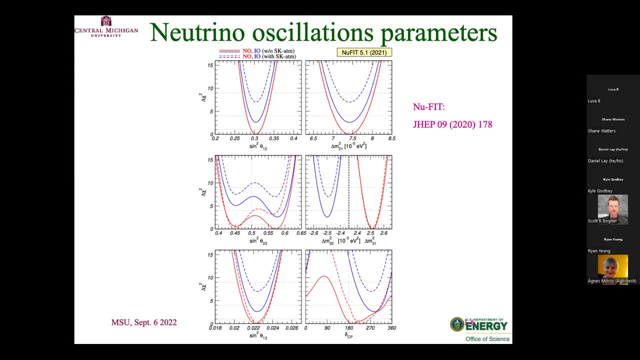 still normal hierarchy is favored, but not the 3.5 sigma. so it depends if you exclude the atmospheric neutrino or not. so again this, the problem, i guess, is experiments, because they are very expensive and so on and so forth- depends on the knowledge of the matrix element, but also it depends on the 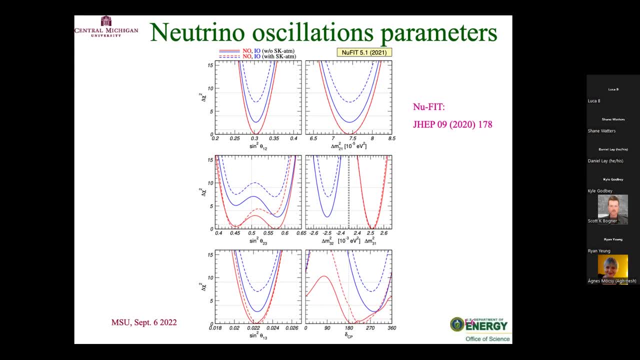 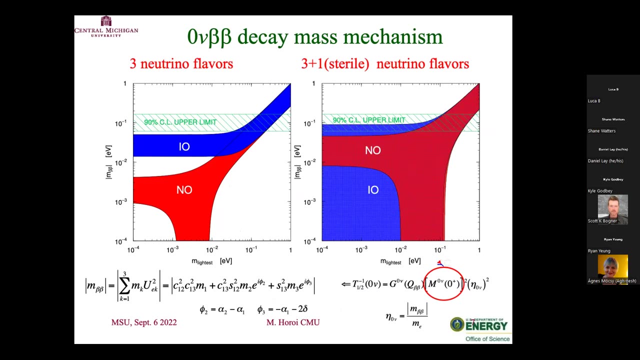 neutrino physics. so therefore, coming to that is: can we help the experiment, can we guide the experiment with some theoretical calculation? and most people are calculating this matrix elements for reason i just explained. also, there is a possibility to be a sterile neutrino, and again for many years. 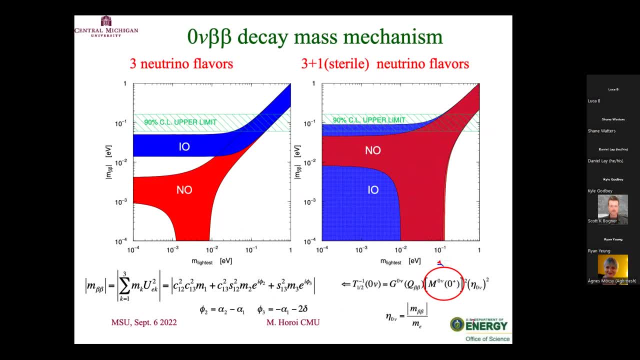 this was favored three years ago as a prl from margon and declaring victory in terms of the experiments come from mini boon. but the micro boon apparently rule out the sterile neutrino. so we are kind of back to a more constrained picture when it comes to neutrino physics. but in the end, remember that there is dark cancellations here. 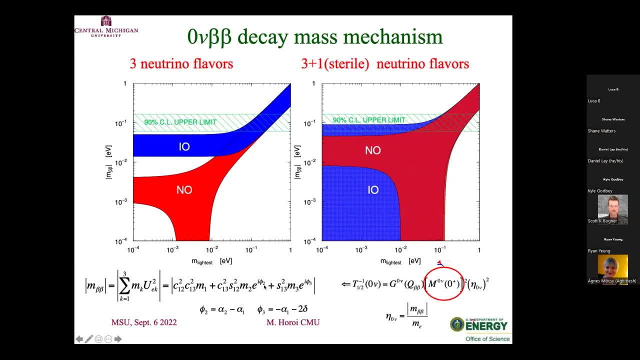 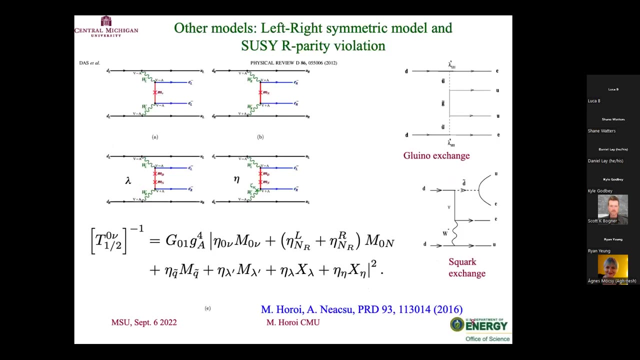 because interference in the in the wake interaction part. and that's not everything. although most people calculate this matrix element- and today we're going to mostly talk about this matrix element- which are related to the mass mechanism, there are many others. so, over the years when no reliable information about the neutrino masses were available before 2000, 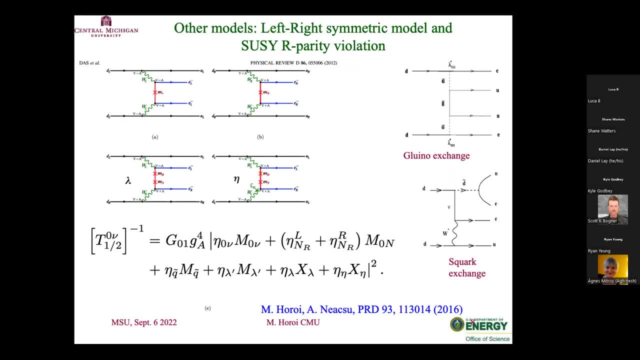 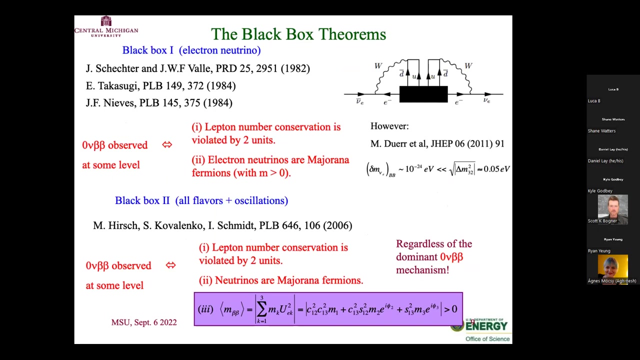 it was just speculation. people will start proposing all kind of other mechanisms, some of them coming from the, and probably nobody see the upper part of everyone right. there will be a problem. can i? is there any possibility to? oops, sorry, i can go back. can you remove it? 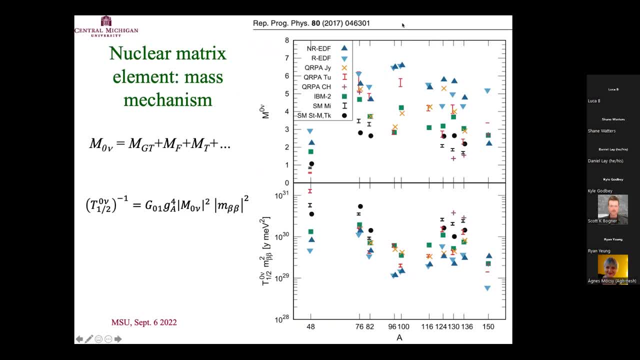 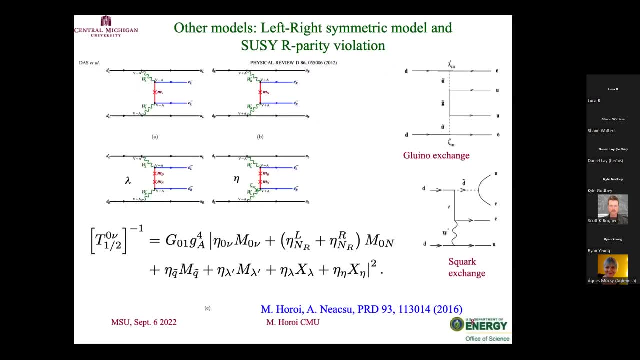 at least the more. yeah, i can't click that- more things, sorry. all right, okay, so let's go back. it doesn't, doesn't appear on my laptop. yeah, it's only on the screen, it's okay. there'll be a little bit of problem at some point, but 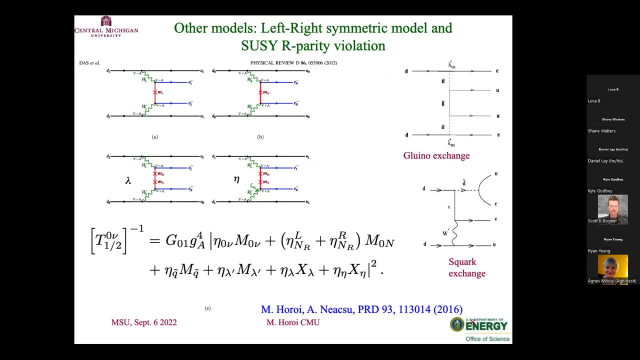 we'll see anyway. so in that case now, actually the the decay rate becomes more complicated. this matrix element essentially is an amplitude which have to get squared, but there are more terms coming from the, the left right symmetric model, which you cannot see. so these are pieces of the left right symmetric model. 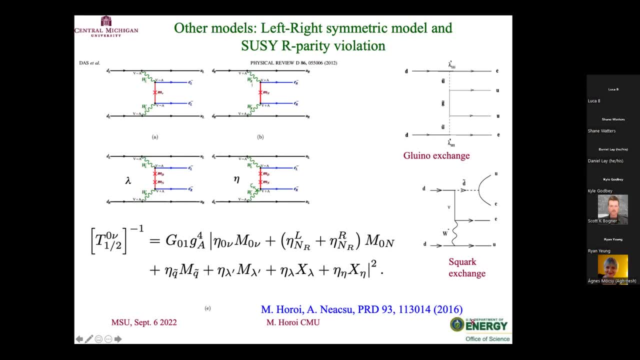 so this is a mass mechanism and there are few other. these are a right-handed heavy neutrino exchange. there's a so-called lambda and eta mechanism. we'll discuss in the 1980s- already later on, the super symmetric models which also are not very favored by lhc. 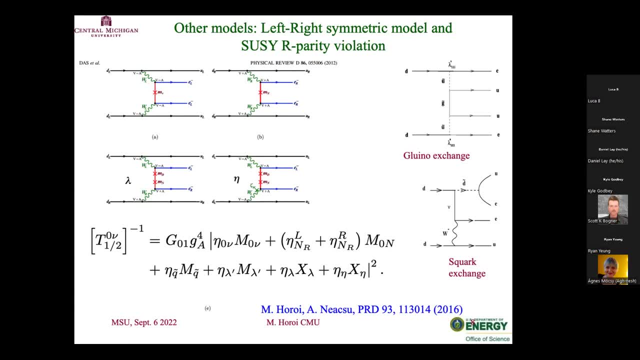 get some green and squark exchange and we calculate those things. so these are coming with matrix element, but it's more complicated because matrix elements here actually are a combination of phase space factor stuff which depends on energy and the and the nuclear structure pieces. okay, so keep in mind that this can lead to interference and can actually cancel everything. 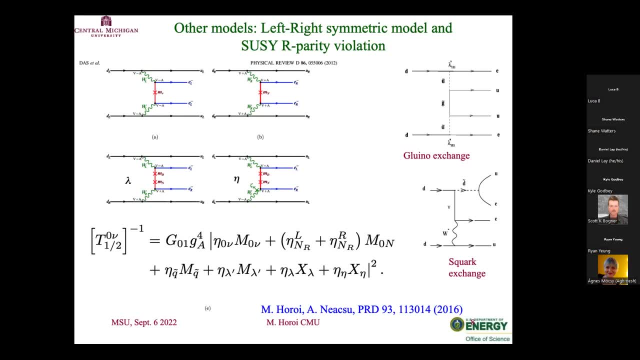 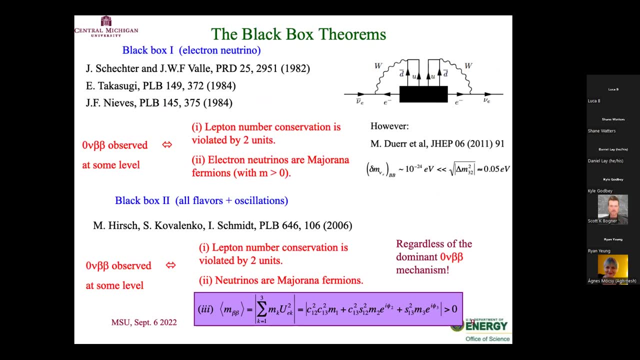 so that's a problem. okay, now, for many years, people uh hail this process as a majorano neutrino discovery, but in fact, uh, neutrinos are well, you can only emphasize the fact that the laptop number is violated. you come from zero neutrino, zero leptons, from the decay nucleus, and you get two electrons in the end. so, um, there's a lepton. 9. 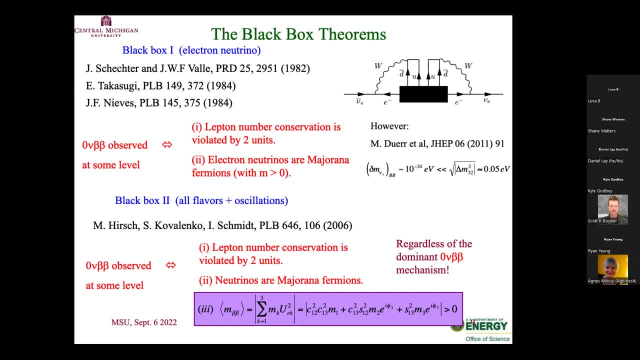 about poz aye volume, leptin 9, lepton number violation. however, people spend a lot of time proving that. in fact, even if it's only a lepton number violation, one can show it at least at some level that, uh, if this matrix element exists, it will imply the neutrinos are majorana, although 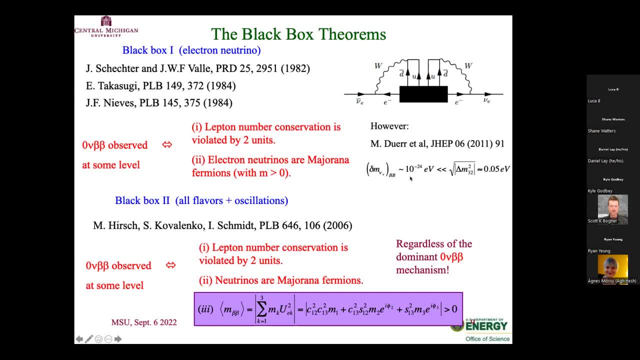 the contribution of this term to the mass is very small, the order of 10 to the minus 24. on the other hand, we know experimentally that, you know, have a milli-electron walls mass gases. so therefore there will be real proof that this is a Majorana neutrino, although 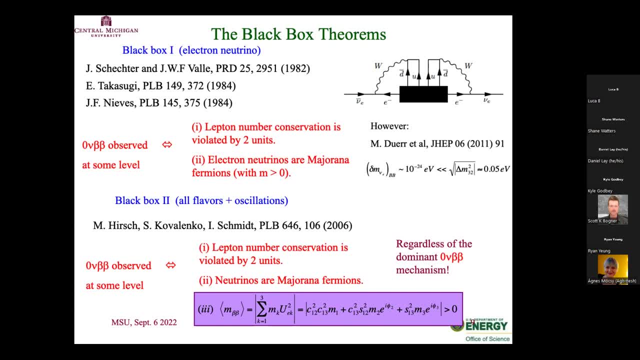 many people are debating that that's the case. So the black box theorem will prove that. okay, if we discover at some, at any level, neutrino, less double beta decay. the neutrino are Majorana. In principle they can be Dirac. 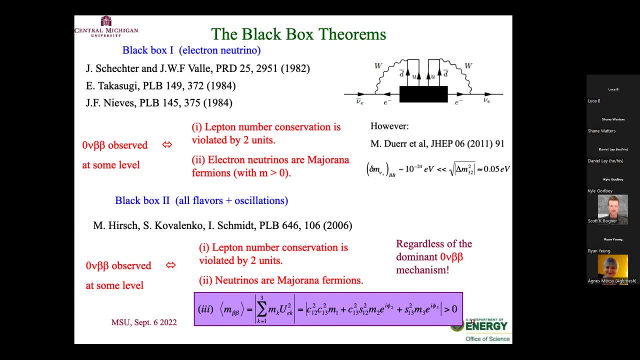 there's no issue with that, and actually that's the main the crux of the problem for particle physics. If they have to extend the standard model, should they add terms such as in which the neutrino are Dirac or Majorana? So that's, at the moment, the right-handed neutrino does. 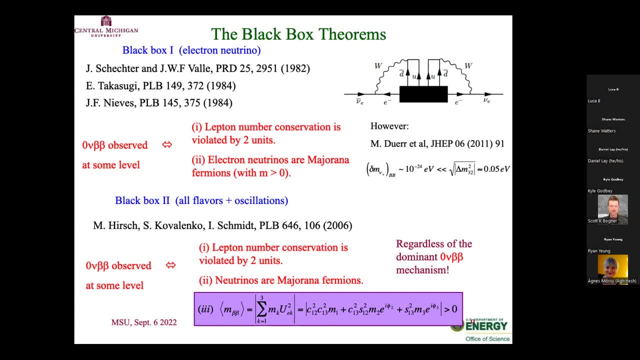 not exist in the minimal standard model and therefore the neutrino in the limited standard model doesn't have a mass. but the question is how to extend them. Okay, talking about that, let's go to the matrix element. As I say, I'm going to mostly. 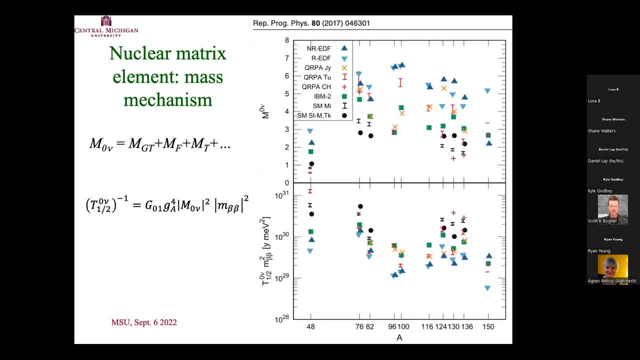 talk about the matrix element. The matrix element for the mass mechanism is a picture from my review paper, which you don't see it here because it's on the top. It is a review paper written in 2017, I don't believe there's any more on that matter recently by John Engel and Javier Menendez, So they 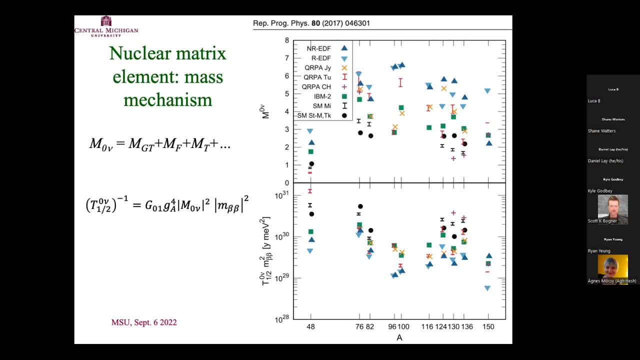 have this overview of the matrix element. I told you the matrix element. actually, they have different pieces which you can calculate and you can control the phases. In fact, the Fermi matrix element is actually negative. So, as I say here, you control the. 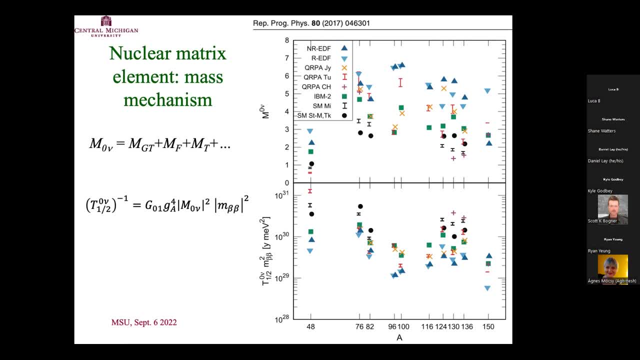 interference. On the other hand, for the weak part, we don't know about the m-beta-beta. So you can see the first. this is a picture which is a little bit democratic in the sense that they try to put all reasonable matrix elements in the picture, and you can see that. 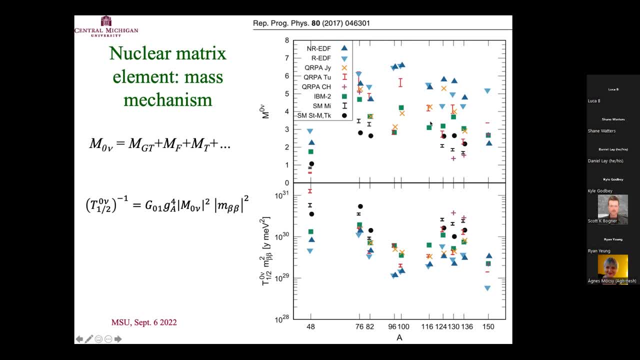 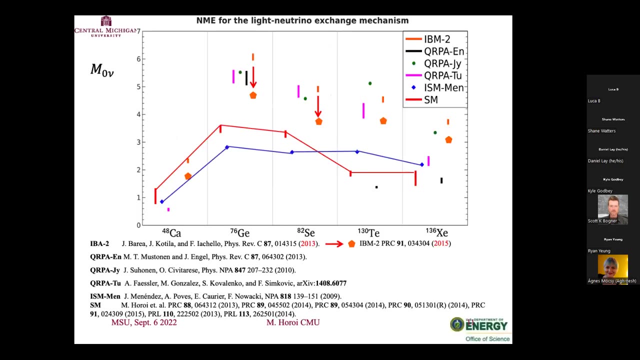 for most of them it's a factor of three to five difference, with one exception. The exception is calcium-40.. Which is easier to calculate here, actually the uncertainties with a factor of 10.. So I made a similar picture some time ago which I excluded because many, many of this. 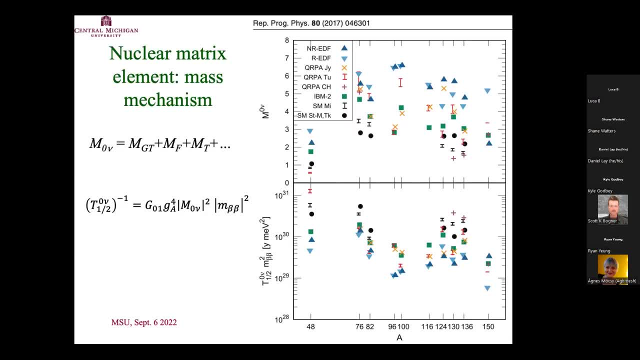 model used here to calculate actually violate a lot of symmetries, basic symmetries like isospeed, number of particles, whatever. They break everything. So I was trying at least to keep those which don't break the isospeed- because that's important- in at least two neutrino. 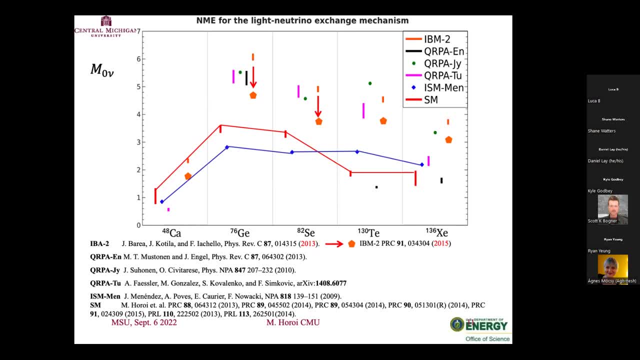 case when you have a gamma of talent. So still, if you look to the heavy isotopes, these are the isotopes which you can calculate in the shell model. There are more isotope than that but for many reasons- like a good model, space and other things, complex deformed cases- we cannot calculate. These are the 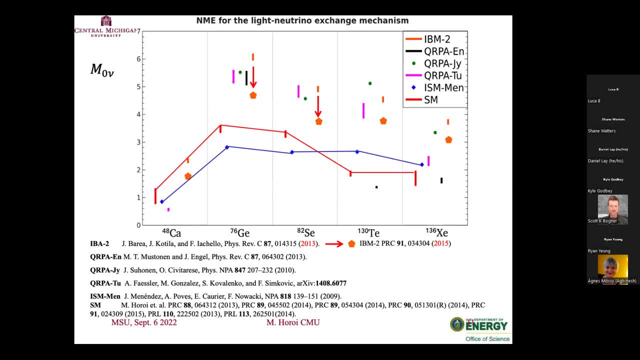 main cases which can do in the shell model- and most people can't calculate their: Beltyim-48,, germanium, selenium, tellurium and xenon. We can also do the pin 124, which is not listed here, but we did pin 140 actually. uh, i got a paper in 344 and got a. 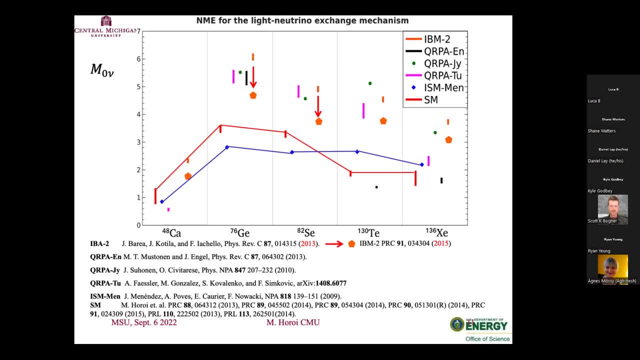 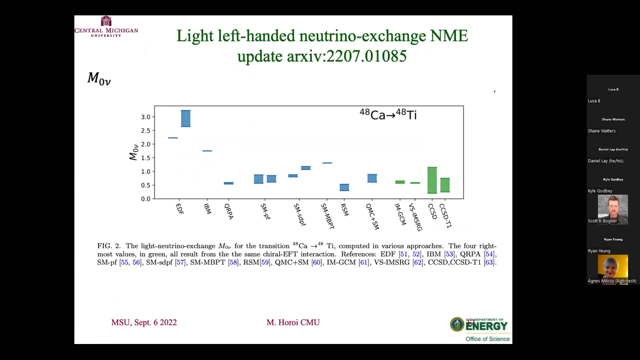 lot of attention. okay, nobody measured even two neutrinos. this also all these size of top people already measured the two neutrinos, okay, uh, half-lives, you can see here there is still this factor of three or so between different matrix elements calculated with different method. so, as i say the the, this is the paper which came out after this workshop, which we have in. 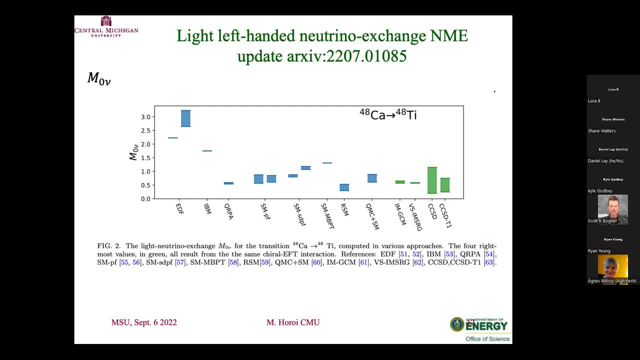 february and this is the picture which is you can find in the, in the preprint which is now in the process of being submitted, i get the general physics g and you can see here are mostly a lot of methods here and again. as i say, if you take this piece and this is a factor of 10 or so, 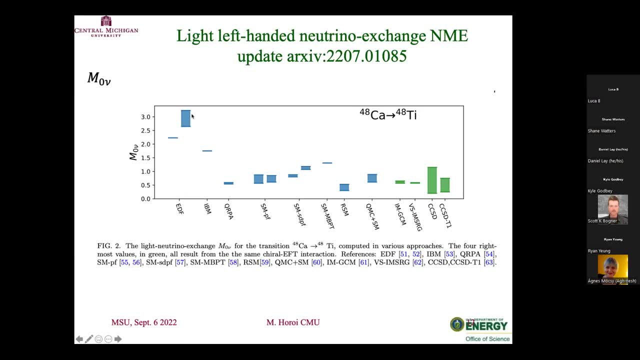 maybe more you can see. here are mostly a lot of methods here and again. as i say, if you take this piece and this is a factor of 10 or so, maybe more, you can see. here are mostly a lot of methods here and again. so it would be nice to find out. 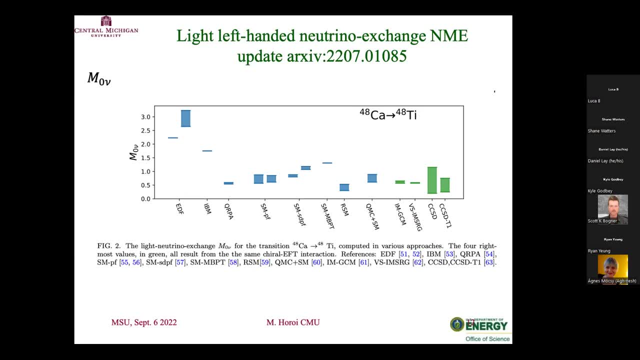 reasonable matrix element and maybe an error on that. okay, so that's one of the goal of this collaboration and again, so keep in mind that here we have a kind of a subjective view. this is a bayesian view, right? so everyone is providing a matrix element and 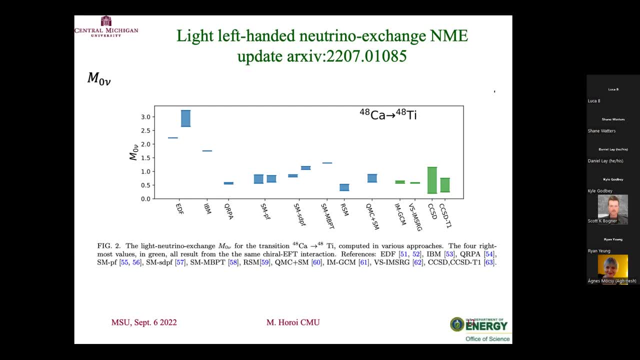 saying: this is my matrix element, meaning that the prior is 100 for that and zero for the others. so, whatever you do after that doesn't really matter. the players are zero for all the others. okay, so, uh, therefore, we decided to do a statistical analysis in which actually, 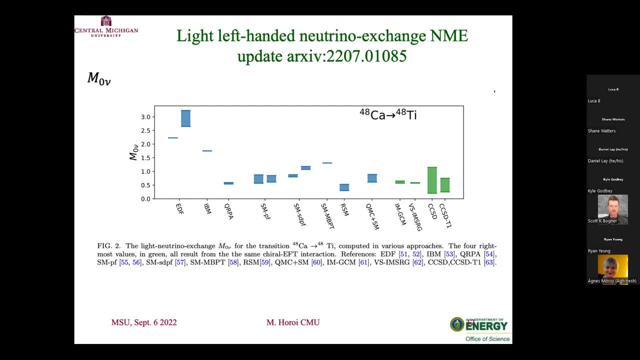 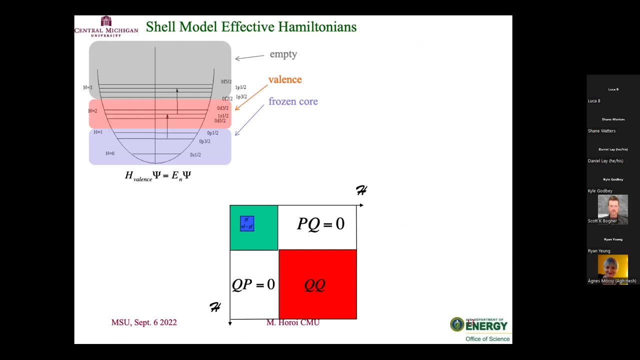 we're going to take democratic priors. in other words, all of them are valid. now, of course, i cannot do a statistical analysis for all these methods, so i have to do a statistical analysis for them, for example, and we'll see how i do this in a few slides. so there we go under the 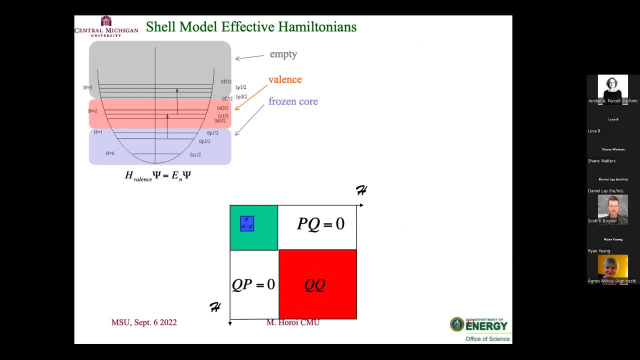 still. we have soikat, we have Winter, is is here. so in the NS один control model we get those. so there are people which are doing like heiko is doing more ab initio kind of stuff, but this is some kind of in the old scheme. the advantage of this is you'll see immediately. 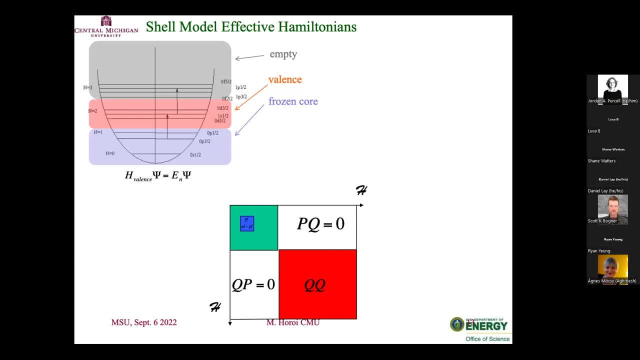 is there are some disadvantages, some advantage that the disadvantages: that this method actually only highlights the energies, not the observable, like transition probability and stuff. but on the other hand it turns out to be flexible enough. it can be described pretty well: deformations, uh, the coexistence of the formation, that a good pairing, and so on, so forth. 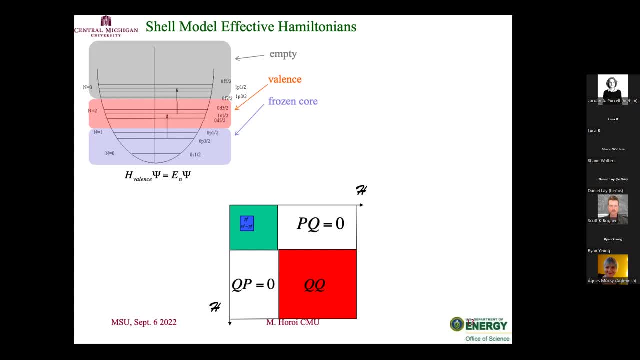 okay, because it's more flexible. so it starts again usually from a yes, go ahead. i'm going to explain. you know that for the moment i'm just starting with a fact that i'm going to use three different starting Hamiltonian, that i'm going to add some kind of. 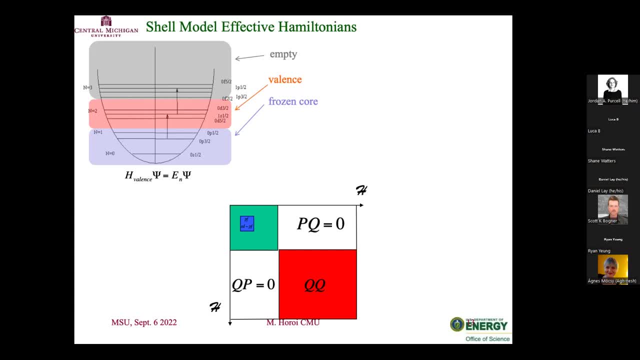 random contribution? no, that. no. each model we're going to have its own thing, but you'll see which one is more important. that's the idea. so there are two things. first of all, you're gonna see how stable is, because you can see- well, that's one of the issues- if you add some kind of random contribution to your input data. your Hamiltonian. 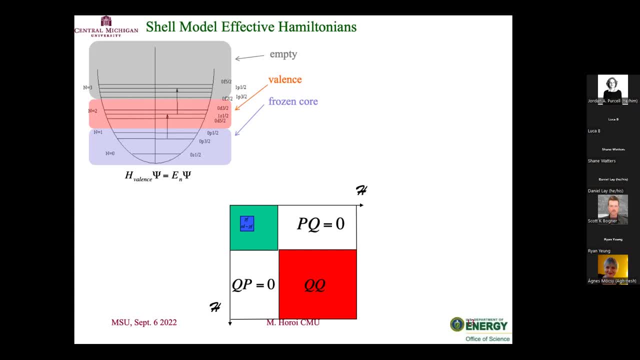 they might actually be unstable and give you all kind of results. and secondly, if i compare several Hamiltonians which are on the market and everyone is giving his own number, which one better describe? and if both, all of them or some of them, better describe what is a common? 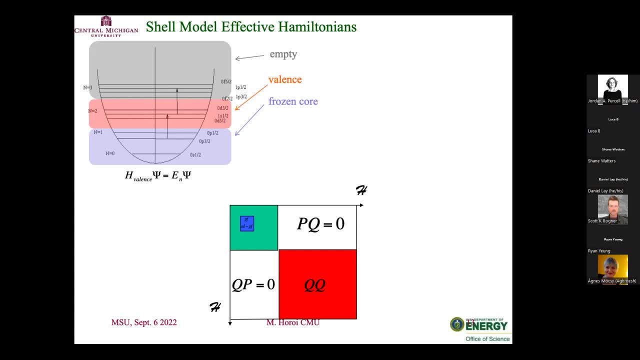 distribution and probability. okay so, um. okay so, um. so the way we do it, we start from some ab initio kind of Hamiltonian, but we can either use a more phenomenal, phenomenological one like the cd bone and after they do some transition to a shorter model space from, let's say, 200. 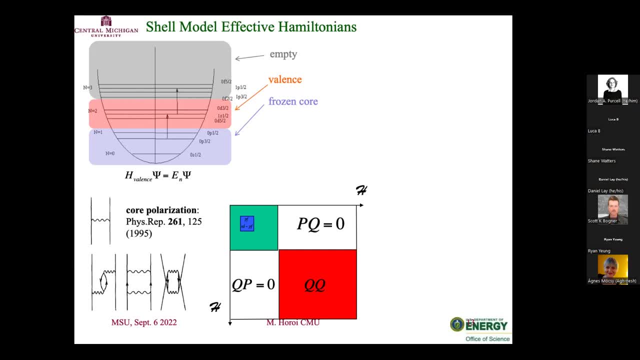 harmonic oscillator shell and do some core polarization, maybe like Morton is doing, or maybe you can use 0k, and after that, depending on your starting point, you start to find out how well it compared with the data. so it doesn't compare very well at the beginning, but if you fine-tune a little bit this matrix element- this is the case of 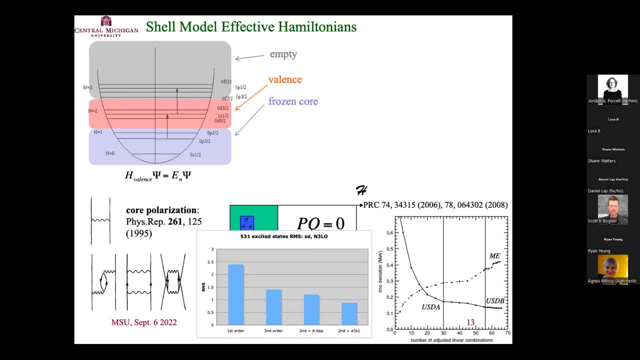 sd. this is from Alex Brown paper about usda, usdb. so essentially you try to fine-tune a little bit your matrix element. they are 63 for the model space which is highlighted here. here and you can get a new sda which is the black line and that's described pretty well. 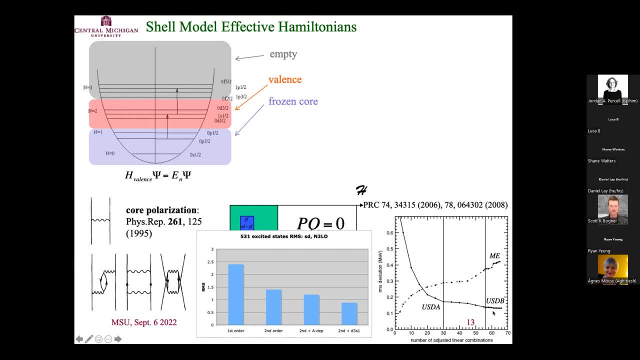 the data, the rms, you're about 500- the excited state energy put here, there is no transition matrix element, including only energies. so in other words, you fine-tune your ab initio, let's say set of matrix elements to the data and the only data here are energies. then you can get. 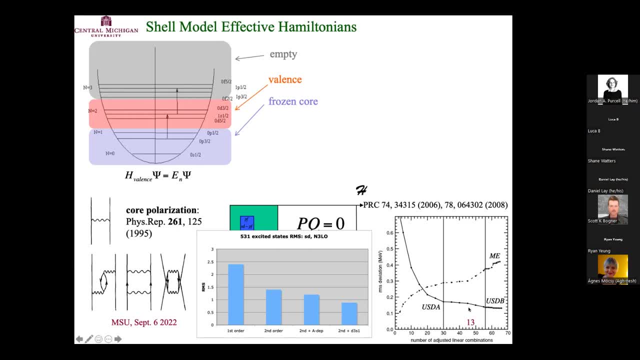 this, and in that case you get something reasonable. the rms go down to about 150 kv, and now you can kind of describe physics: if you overfit, you go to sdb. in that case what happened is that you don't get anything good, much better. so it might go down to a little bit better rms. 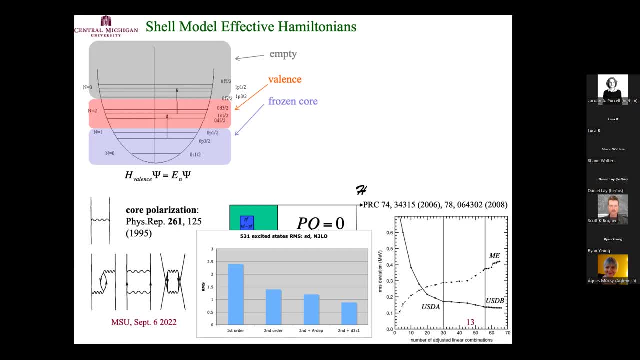 but your matrix element will be more different from the original. and that's a problem because when we calculate transition, we depend on couplings, on phases coming in couplings. so it might happen that you, in other words there- are unitary transformation of your single particle wave function, which we're gonna essentially destroy any observable. you calculate because 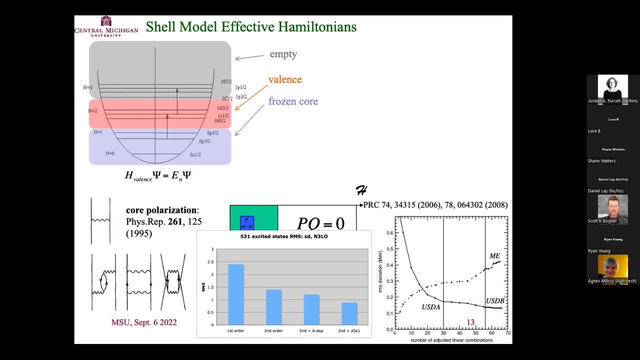 if you change you're gonna get good energies, but but different phases. so it's not a good idea to overfit. so in general we do a little bit of fine tuning, but no overfitting. so with that we get a good energies and the outcome is we describe. 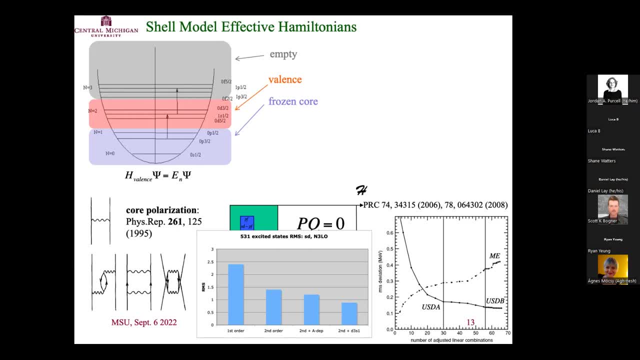 pretty well. we could describe energy. we're going to describe better rotational spectra, collective states and stuff like that. when it comes to observable, there's a problem all the time, and the problem is that, although there is a kind of one-to-one correspondence between theory and experiment, like in 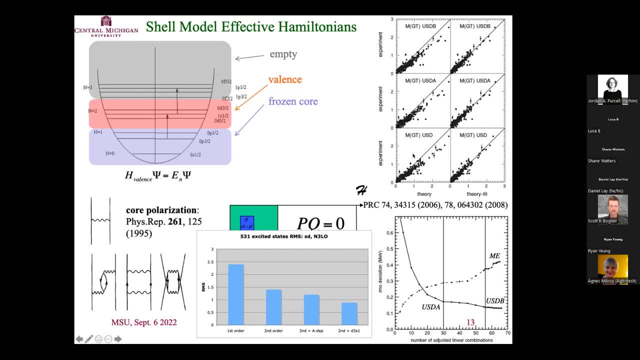 the first column here and it's not on the one-to-one line, right? so in order to get a one-to-one line, you have to find something, and the simple thing here is to use a quenching factor, right? so in other words, here in general, people look like in different ways with it, like the. 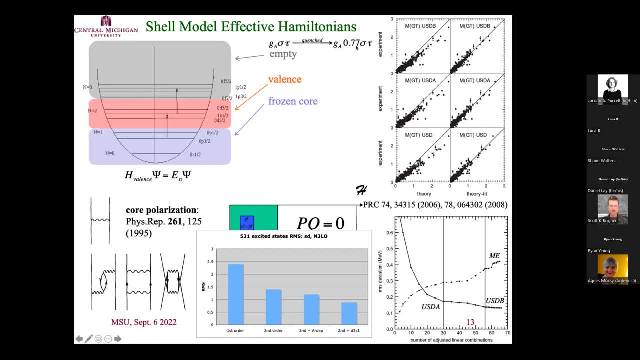 ga is quenching, but in fact, there's no ga quenching, it's just the matrix element which is quenching for the gamma of teller. okay, so that's a good part, but it also is a good part. but it also is a quenching for the gamma of teller. okay, so that's a good part, but it also is a. 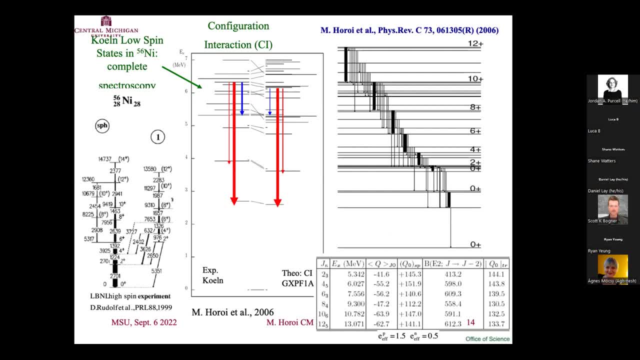 we can describe this. this model described very well collective things, even for this complicated nucleus like nickel 56, where we have- essentially, it was said there's- a double magic nucleus. it's spherical, but at about five amygdala is a super deformed band and everything is described very well. 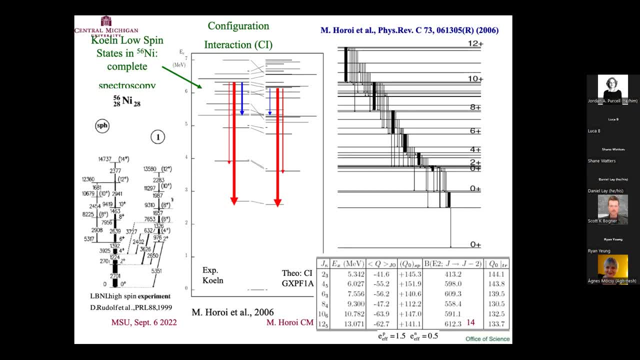 without anything extra. okay, and we can describe the energies as being a rotational band and it can also look to different collective major measures like quadruple number b2. they are all consistent, so there might be something here. okay, we might be out on something, even when you describe observable. 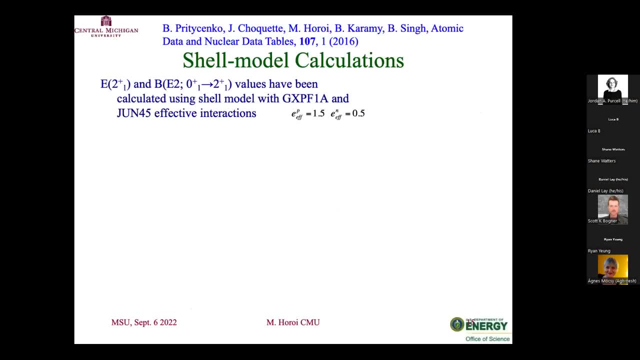 and also we have. we for the b2, we have to use this effective charges. that's another downside. so for each of this operator we have to adjust them a little bit and we adjust it in a simple manner. if we do it more complicated you might get better or some, some nuclei, but worse on the other. 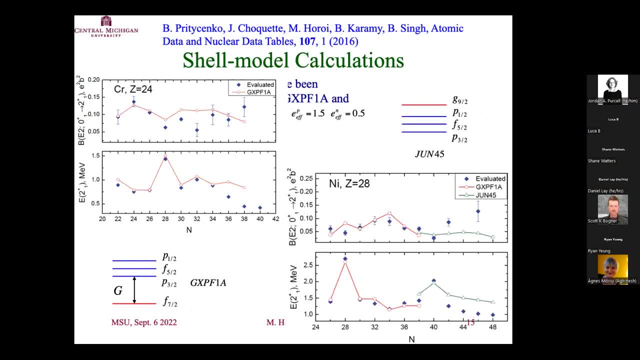 so this is a some results in the fp space and the one which is called jj44 and we can see that actually describe reasonably well the two plus energy in the b2. the b2 states: okay, so this was the, the first part and the, so now i'm. 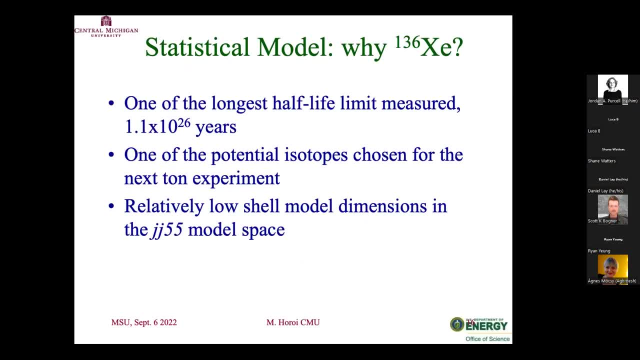 going to talk to more about a statistical model. so why do we want to do a statistical model for xenon? okay, first of all is one of the more uh thought nuclei. in the case of neutralized diabetic decay experiment is one of the highest half-life limit measured and there 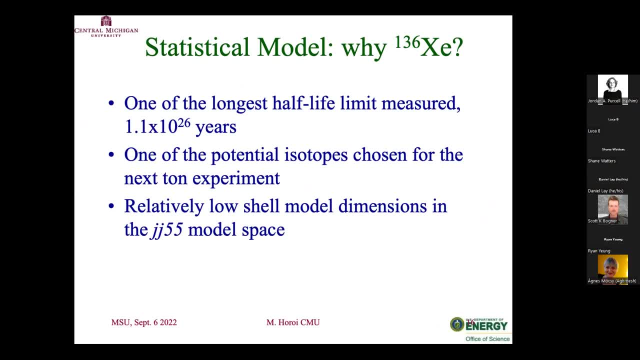 is obviously still a debate. which isotope should be funded at the tone level will be either germanium or xenon, so it's an important one. in addition, it turns out that, although is a heavy nucleus, we can. we can actually the shell model, the sozusagen curse, a wave nucleus is going. 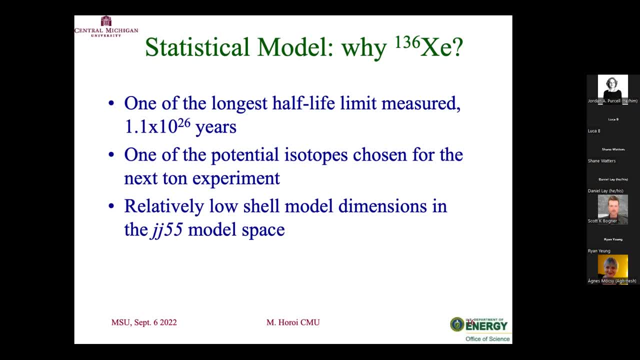 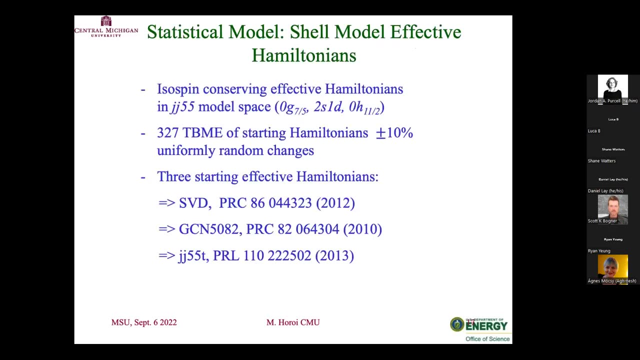 dimension are not extremely high. that is more more involved calculation than calcium, but it's not like germany or you know, or tellurium, stuff like that. then uh, so the, so, the um dimension is relatively small, okay, so, um, so we're gonna use, as i say, um, uh, isospin, conserving hamiltonian. 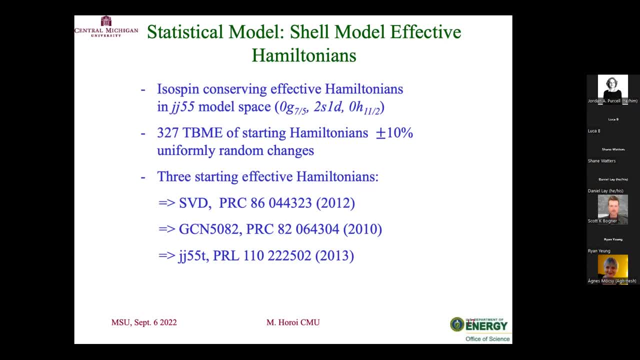 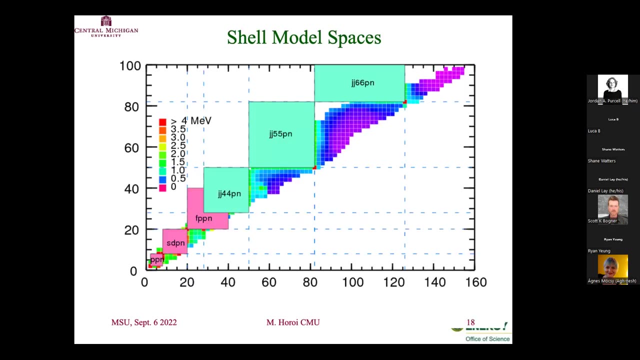 three of them, the model space uh, have a funny name. we are physical physicists. they are not good giving. i believe this is alex uh naming jj55, because there are five states here. there are two d states, one estate, one h and one g uh, it looks like that. so, so it looks like. so this is. 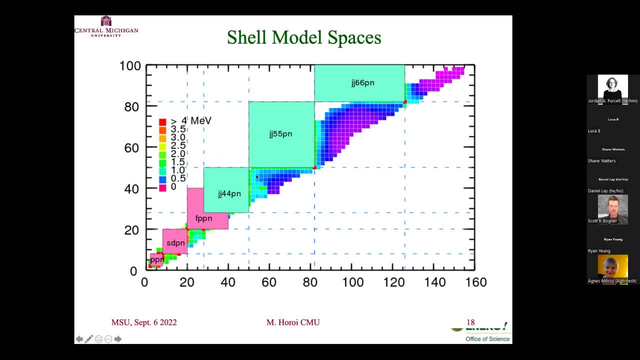 uh, this piece here and we are in this corner. so, in principle, when we have a model space, you have a core. you may say the core is still 100, but in fact the core is still 132 because they are going to have uh, proton particles and neutral holes. 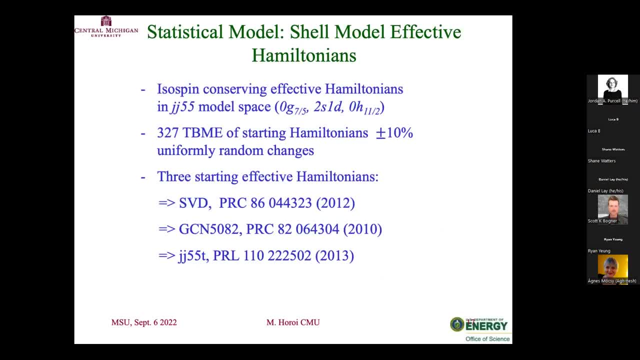 all right. so, um, uh, there are a large number of two body matrix elements- there are about 327- and we use three starting hamiltonian. each of this hamiltonian starting with their own scheme. they start with g matrix will okay, and after they do, fine fine tune for certain data. for example, 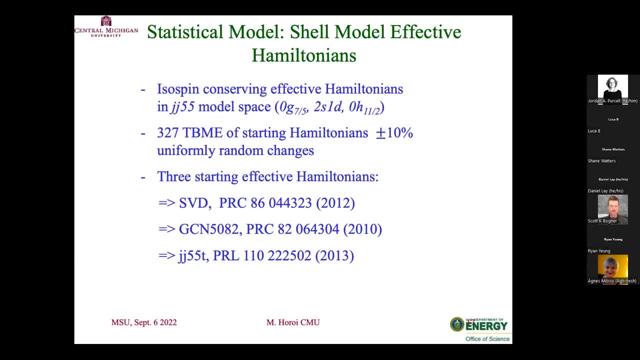 g, g, c, n, 50, 80, 2 is one of which give you very good energies, was just fitted for many, many energies. svd was mostly fitted for uh, tin isotopes. so therefore mostly the t equal one matrix element or effective and that have a. they have a good upsize if you don't change too much your matrix element. 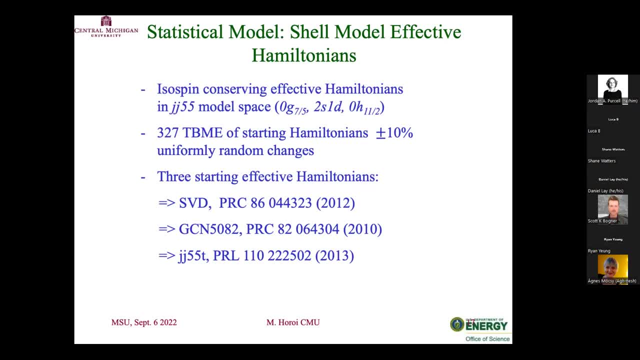 you don't run the risk to change too much your matrix element from the original one. so in terms out that svd. actually you don't need a really low quenching to describe gamma tellers, so gcn need a quenching to describe the two neutrino matrix element, which is about 0.35. 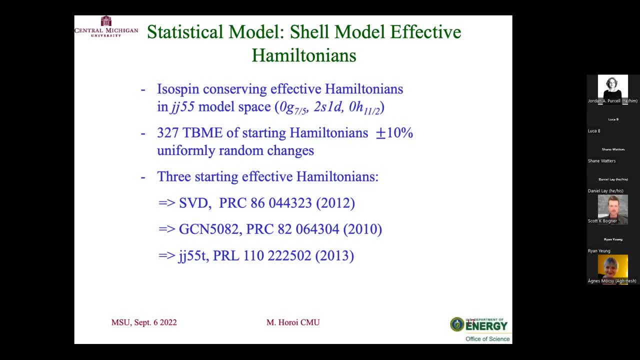 rather than 0.7, and svd doesn't need that. jj55t is the stuff which me and alex used for describing in a prl. the zero and one thirty six is something which changed both. also the t equal one and t equals zero two body matrix element. but uh, it's not really overfitting, it's just a fixing, let's. 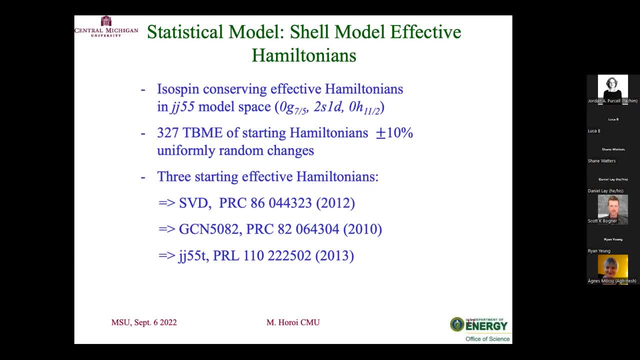 say, we try to be mild, fine tuning things rather than overfitting. so these are the three models, right? so the first thing is to see how, uh, how reliable are each of them. uh, two changes, okay, and the changes i didn't describe, but based on the 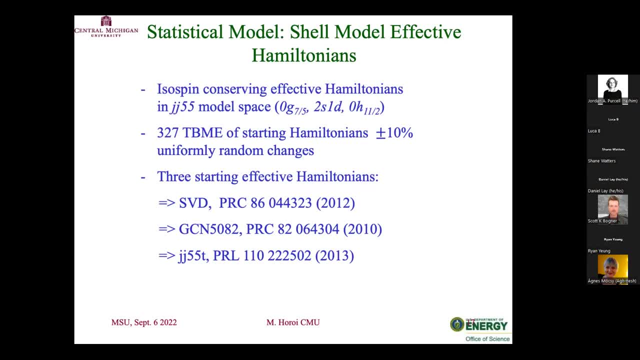 usda. usdb picture show you. i conclude that, uh, if i have to do an overfitting will be an extra 10. so this is your choice. you can choose 10, you can choose the uniform. uh, addition to the starting hamilton. so if these three starting hamilton here we add about 10 to uniformly, random changes. 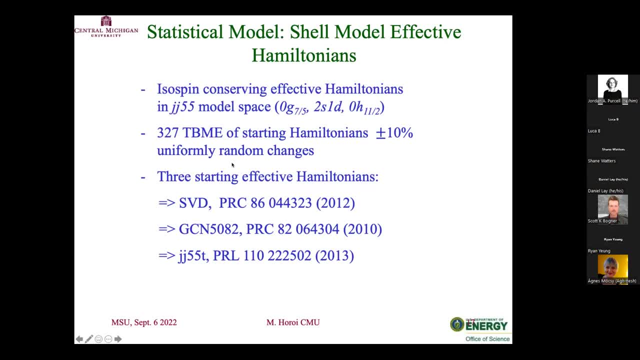 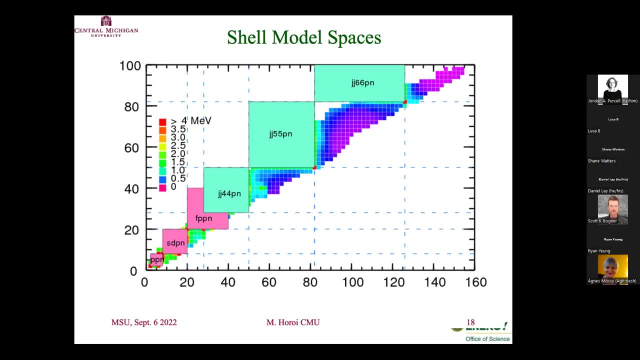 that's what we do. that's these are the three models. yeah, right, okay, so these are the main uh. sinks lc. so this is the okay. so now what's uh? so when we want to do a statistical analysis and you want to favor or disfavors, you have to test your description on data. so what kind of data are we using? 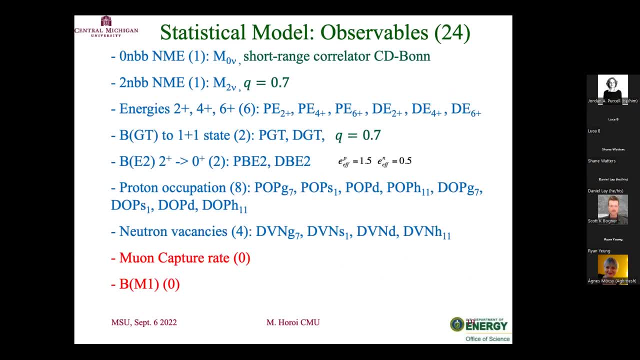 so here is the data. okay, there will be a problem at some point, okay, so, um, so you don't. okay, actually you can see, uh. so here are the data, the data we are using to test the model. they are the two neutrino uh nuclear matrix elements, and here we use a quenching factor of 0.7, uniformly for all of them. 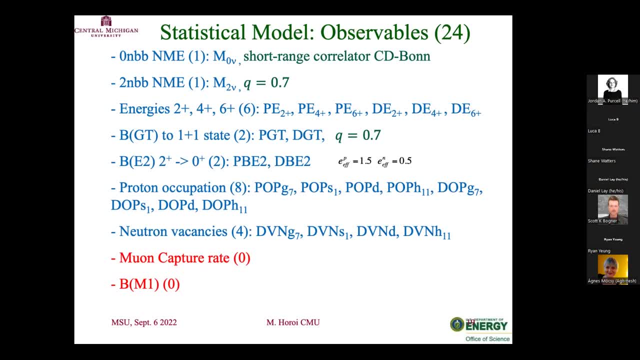 yes, go ahead. yeah, we'll fine-tune. yeah, yeah, yeah, so you don't need to beat this. no, no, so we, no, we try to figure out if we do random change when you fit, you don't randomly move the Hamiltonian, so there is a procedure. 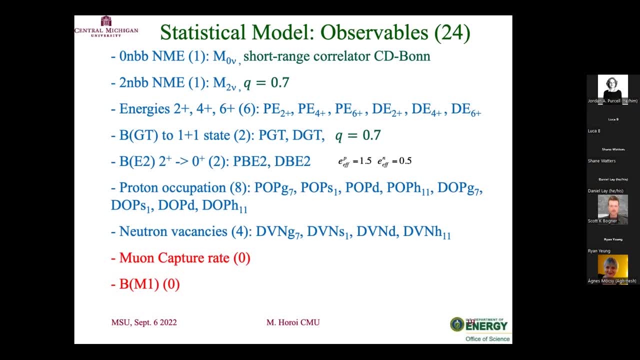 like, let's say, minimizing a chi-square, for example. so we take that and we add in them. so decision was: how big is the random term? so, as I say, I don't want to change too much the matrix element because it might imply a change of the phases and we're going to destroy the 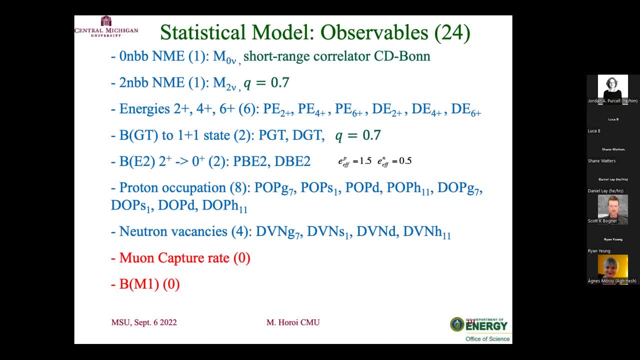 the transition probabilities. so, based on the experiments experience we have from usda, usdb, I concluded that 10 percent will be enough. but I'm not saying that that's in principle. people will think about: oh, I can use any and I can put some weighting factors, which we do because we 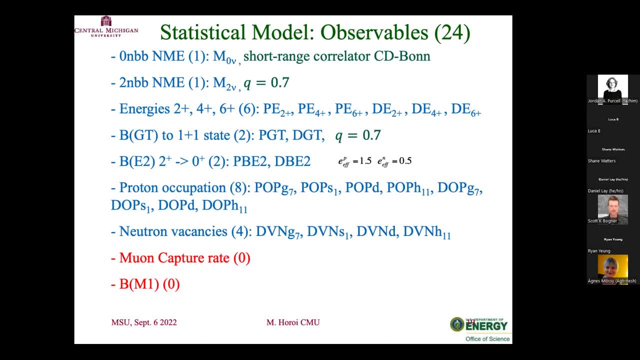 compare experimental data. so there are three different Hamiltonian. they gave me three different matrix element. you're going to see them, okay, so here there is only one. the number counts. the total number of observable is 24 in our case, so of course the neutrino less. 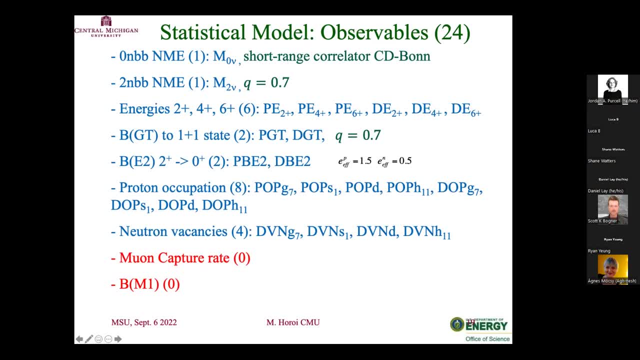 nuclear matrix element is what we are looking for. I'm going to come back to this short range correlator in a while. so we have energy for energy. we don't need anything because the energies are already part of the standard shell model. there is no quenching or anything. there is nothing effective there. 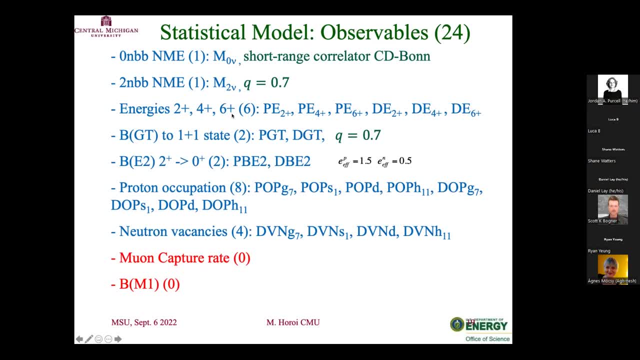 so we look for the two plus four plus six plus put the parent and the daughter. there are six of them. we use the gamma of teller to the first one, the one state I forgot. this is the first one plus state in the intermediate nucleus and this is for the parent and the daughter. when you see the p in front means 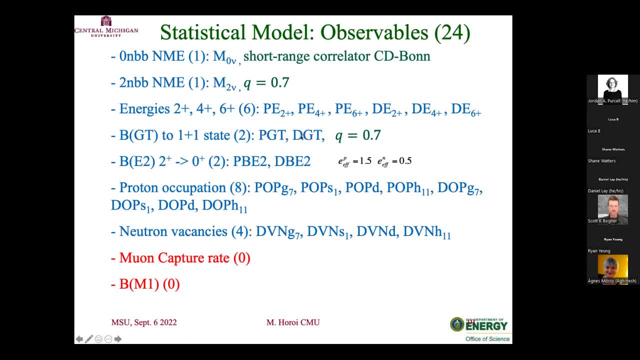 a parent and you see a d is a daughter. because you have to differentiate that. then again I use the same quenching factor as a gamma of Taylor. the two neutrino also is a gamma of Taylor product. so I have to use some quenching factor and 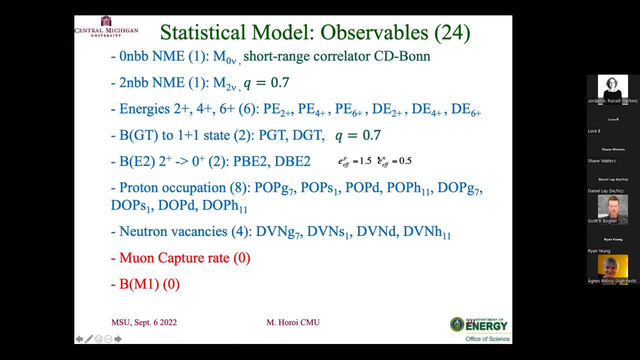 we use B2s, from the 2 plus to 0 plus, and we use occupation for the protons and for the neutrons, because I told you, for the neutron we- actually the experimentalists, provide vacancies, so we use vacancies. It doesn't really matter too much. So if you look on, 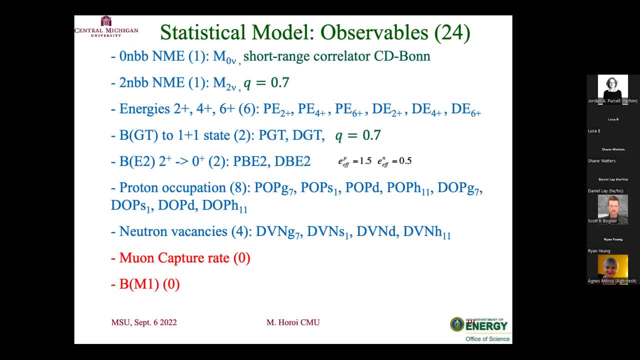 our paper coming from the workshop. there are some other things people talk about: Muon capture. Muon capture is a low-energy muon which is captured by a nucleus and emits a high-energy neutrino. and because the mass of the muon is about 100 MeV, you get the 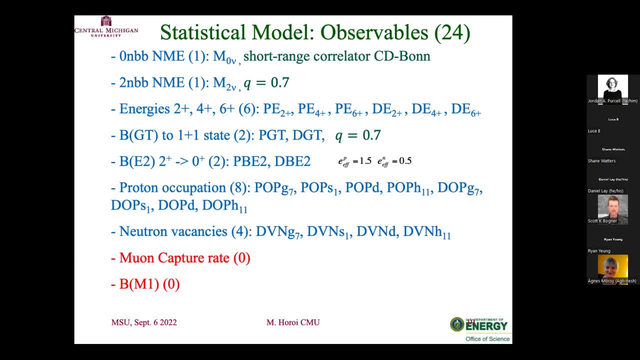 principle, in some cases neutrino of 100 MeV. The problem is again: the experiments are complicated because in most cases a few neutrons will come out, not only a neutrino of that energy, and people may claim that because about 150 energy virtual neutrinos. 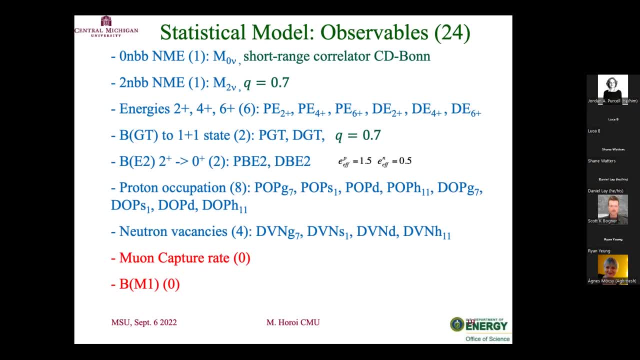 are involved- I'm going to try to argue otherwise. and also people use- I didn't use any zero, So BM1 also are mentioned, but BM1 usually in this nuclear are mixed to E2, so the additional complication plus I have to take care about more effective charges and stuff like that. 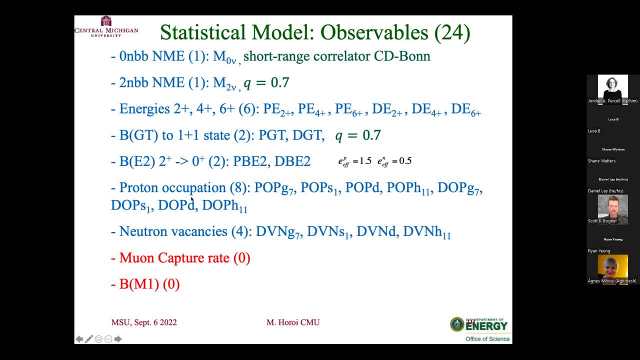 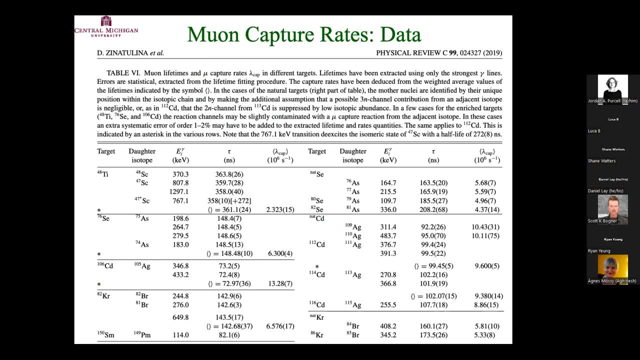 So we exclude this too, because the gamma filler will already capture that. So, for the muon capture, this is the legacy. This is the latest data I could find. So you can see, zero is not on the list, And even if it was, because calcium, it is on the list. but you'll see that actually it's very complicated. 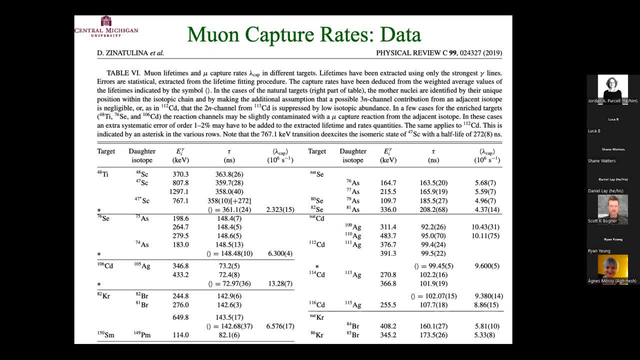 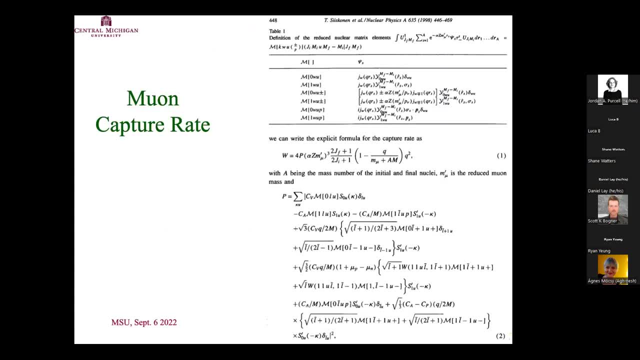 because they have to find the partial decay rate for that. because they say: most case is like a background, Most cases you're going to have one or two neutrinos. In addition, there is this problem: This is how is calculated. The muon capture rate is complicated, It's. 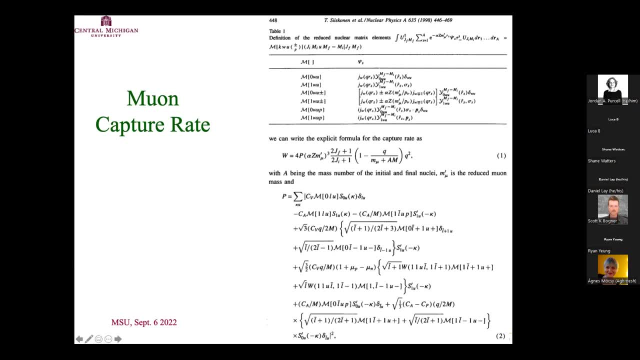 essentially has an additional gp here. but it's not all. that is a long lot of amplitudes which are mixed up and the chances of having bad the interference is very high. in fact, people which wrote this paper which is listed here, you don't see it is. it's a nuclear physics. up in the top is 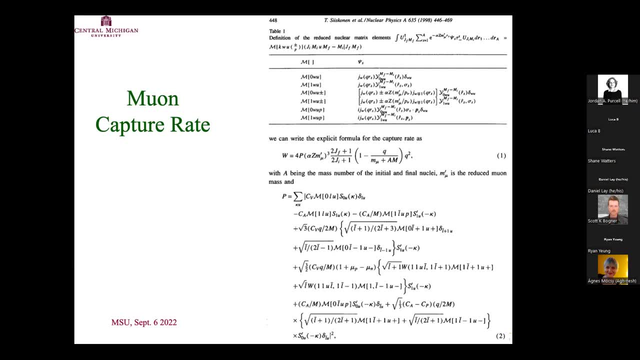 by a so-called group and they they agreed that this was done for light nuclei like official nuclei, and in that case they actually different. Hamiltonian gave completely wildly different results because of the cancellations coming here. so you have to stay away of cancellation. even gamma of tellers. so i show you this point seven: there are a lot of gamma of teller charts, small. they 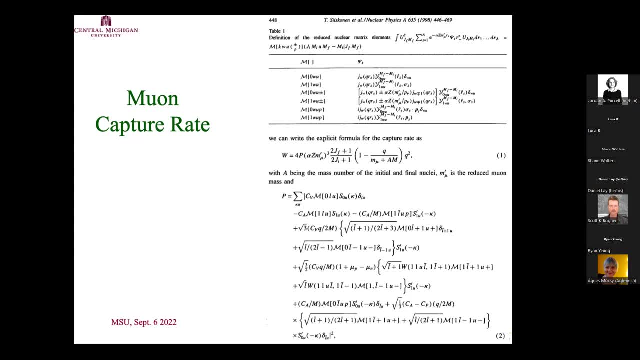 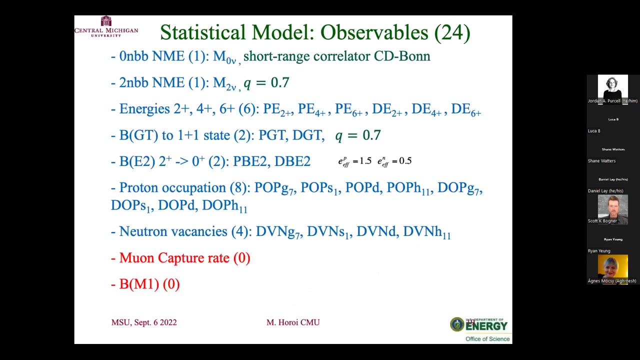 come from cancellations. actually, i can only change a little bit a single particle energy and i can change the gamma of the level of the term relatively easy. so everything careful is cancellation. when you appear, only one matrix element is dominant. that might be okay. so these are the data again. so you're going to need to remember these acronyms here because in 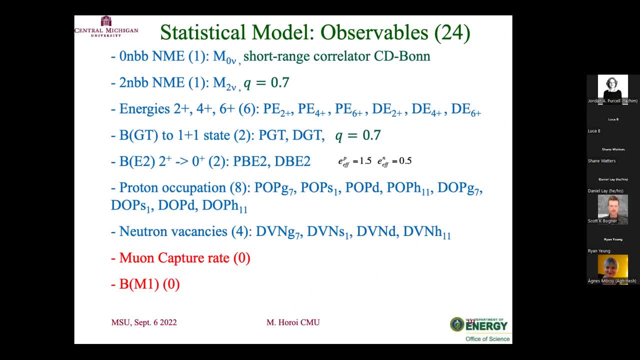 the next three slides, which are the results. the next four slides are all the results. after that, i'm done okay, so there'll be some acronyms. so this one is really easy to look because these are just matrix elements which couple two nuclei: the parent and the daughter. 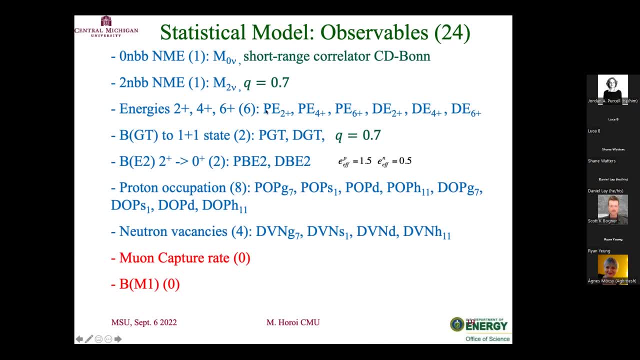 but all the rest have a p or a d in front, meaning it would signify parent or daughter. so you have the energies, you have gamma of tellers, you have b2s and you have occupation of a. so now we're going to be come the complicated part. so i'm going to. i put it again actually: 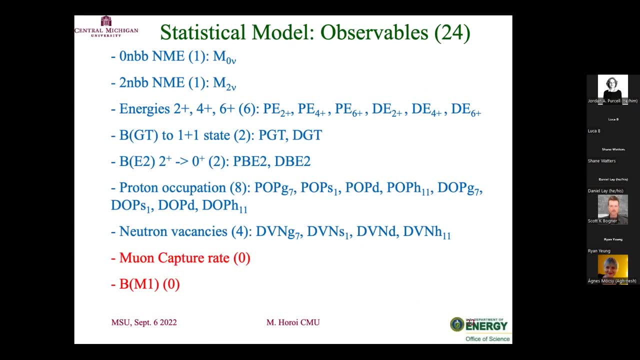 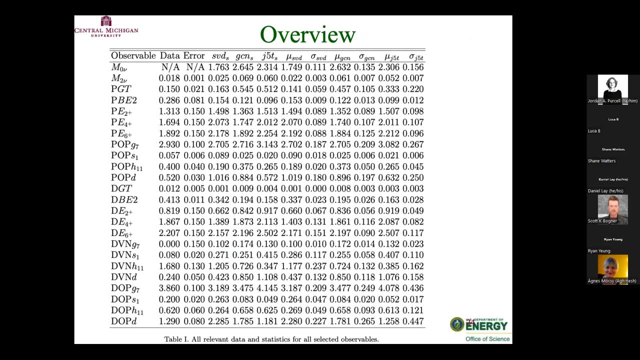 here, just in case, that 24 in total, because i exclude the one in red. all right, so these are the overview of the results. you're not going to see anything. of course that's not. the purpose of that is just to give you. this are the 24 um. 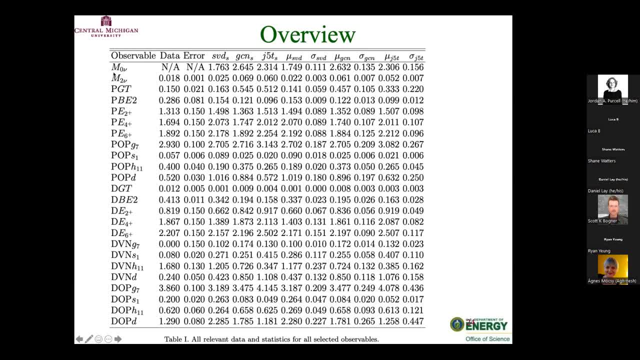 observable here. of course there is no data for the neutrino less there is data. so the whole point of two columns are the numbers that come from the data. that data, okay, so of course data. you know they have some errors. if you look even to the two neutrino decay, you've got to be surprised. 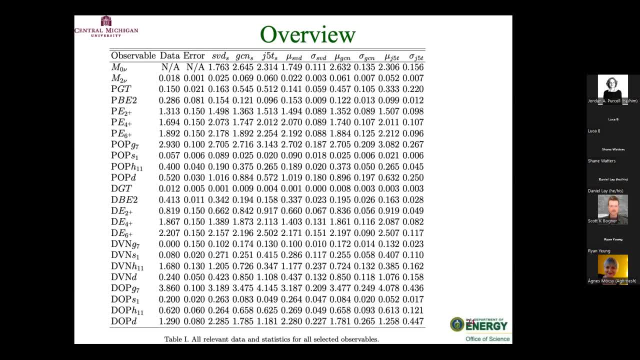 how they calculate the errors. they have pretty much same thing. actually, they are different measurements. some of them measure 10 events, some measure five, some measure 100, and someone have a bayesian way of figuring out what would be the final value. so we're going to try the same thing. 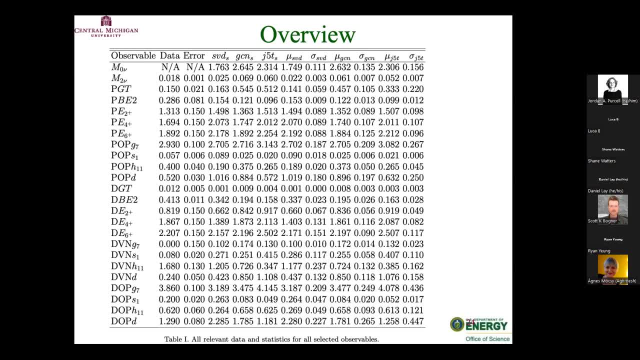 like any good experiment, it's still going to have three models, because people, as i say, normally we use a bayesian point of view. we say our model have probability, prior one and the rest are zero. so we can do whatever you want and we're going to change that. so the experimental is what they do. they take a range. 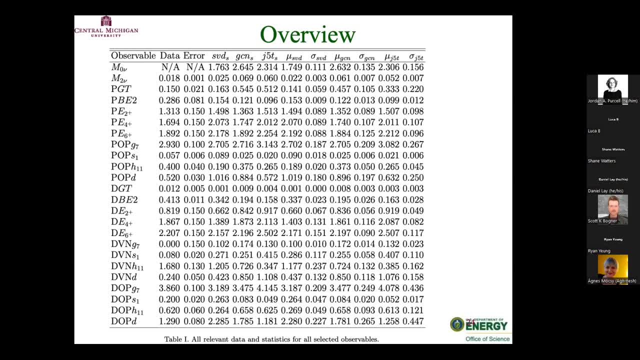 but the range sometimes factor of three, five or seven or ten, so that's a problem. okay, so the good part is here. for each model, each one can do its own statistical analysis. so we can see here: uh, you have svd, gcn, g5t. i make it short and you can, you can find. for each of them, you can find the. 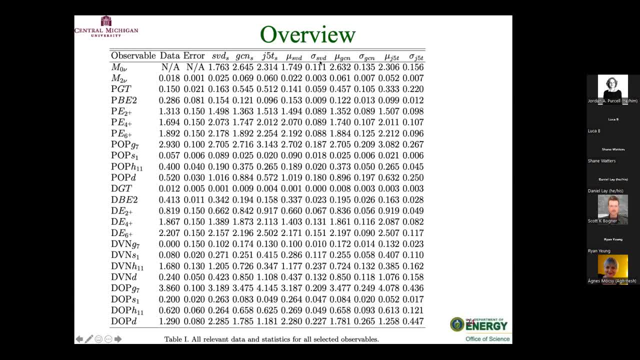 average value and the sigma. so the distribution it's not. you're going to see the distribution, i'm going to show them to you, but you can calculate for each of them and have a big table here. okay, they'll be in the preprint, of course, going to appear soon, but probably another. 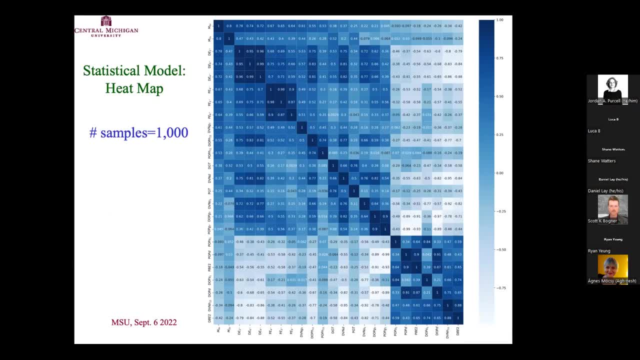 complicated figure is a heat map, so we took here about 100 samples for each of this interaction and they're correlation. actually they're strong correlation. you can see the numbers, yeah, and actually probably you should look up here. you're going to see which one- 0.8, right? so this is the 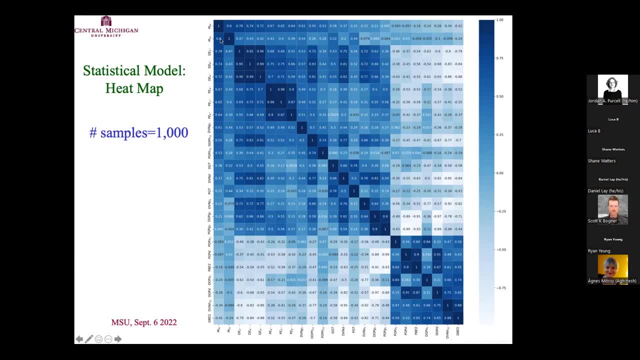 two neutrino, and after that you have the energy, the two, four, two plus four plus and six energy in the daughter right, and after that you start having uh, uh, some uh, occupation probabilities and after this, stop. you can see here, if you look on the correlation, the first column here, everything. 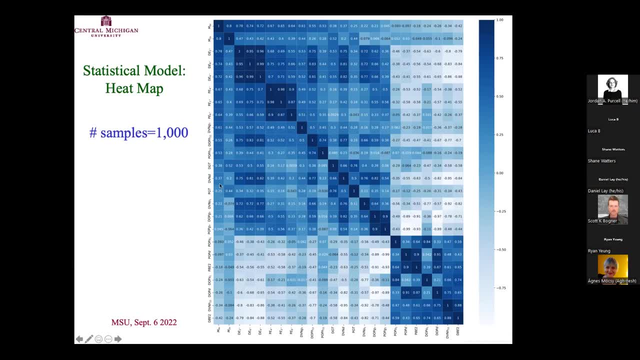 stops about. here is this 0.5- uh sorry, a little higher, i cannot see on my. so this is a 0.55. this is the correlation coefficient and they're also correlating around themselves. so i believe this is actually this. probably this is the latest occupation. after that you get 0.38 and so on. 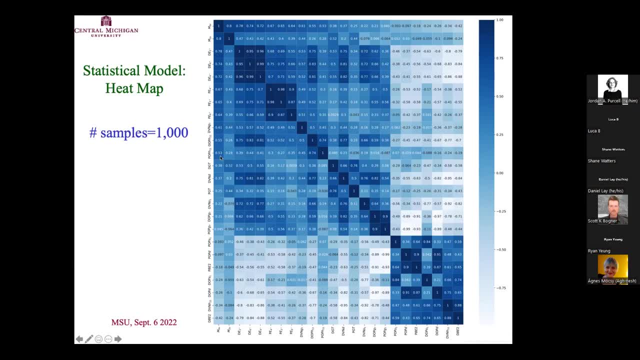 so we see that the two neutrinos strongly correlate into the neutrinos, but after that only the energy in the daughter, not the energy in the parent, because it's a semi-magic. so two plus four plus six plus, uh, and interestingly the gamma stellar is not very. 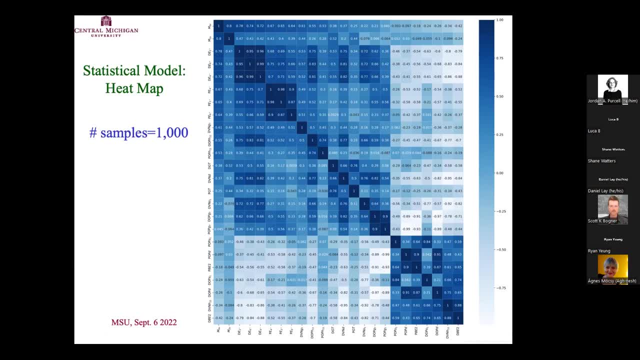 correlated and also the b2s are not correlated, not even b2 in the daughter. so it tells me that actually, because this is close to us, that the daughter is barring 136. so 2, 4 2 plus 4, four classes and six plus energy are strongly correlated, but not the b2s. so you may, you may. 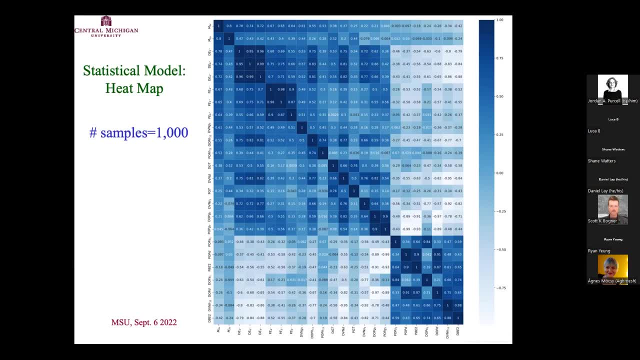 think that this is a little bit deformed, so there is a little bit of rotation, but this, this rotation is probably overcome by the parent, so the pairing is dominating. the mismatching pairing is the one which is dominating. okay, so this is one picture. let's see if i can go to the next, because these 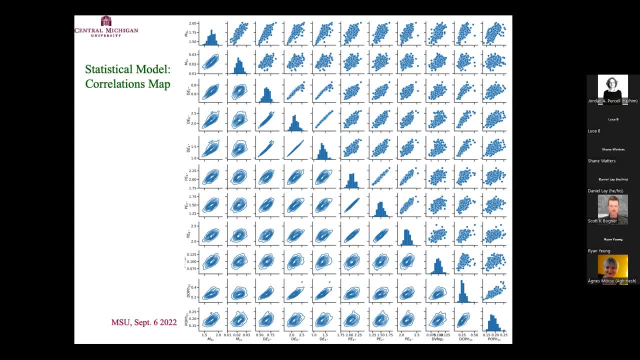 are complicated tables, so this is another way of viewing things. so again, so, uh, you can see, you can. on the top is a neutralized matrix element and here you see the kde on the diagonal, and here are the correlations, right as far as going. they're all correlated and i stopped. 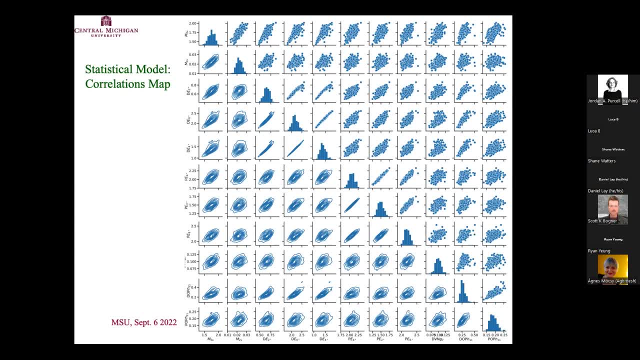 somewhere right here i put only the one which have a correlation coefficient larger than 0.5, so you can see there are strong correlations between them and you can see how they look like. so, coming back to filomena's, you can, we're going to look at that. so you see, these are the 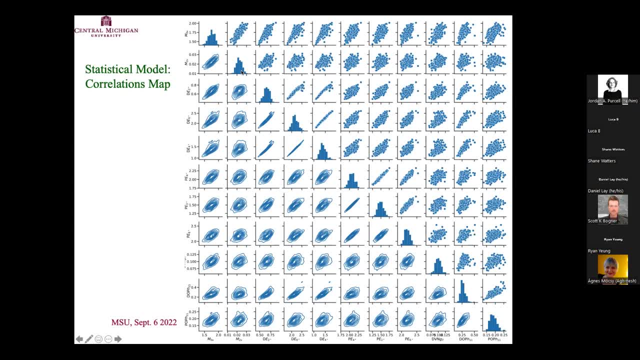 distributions. these are your kde. uh, you know, kernel distribution estimator? uh, they don't in most cases. don't go too far away. the only exception is gamma of taylor, which i don't have it here on the on the list, but these are not all of them, it's only which goes. i'm stopping here- like 0.5 correlation. 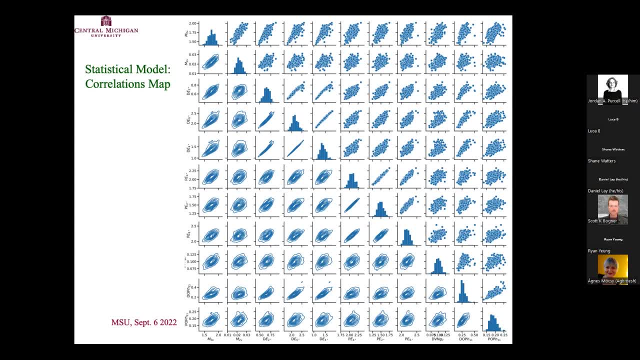 yeah, they're all observable. all of these are the observable in the list. i mentioned that you, that you can see it on the bottom here. right, so you have the. you can look on the bottom because you have the same on the bottom you have to see, so you can. i can explain it, but you can see the. 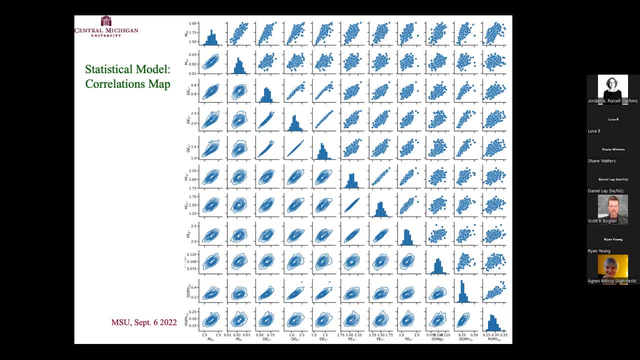 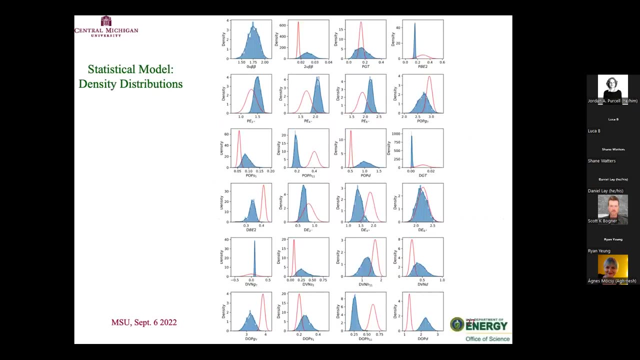 first one is the two neutrino is strongly correlated, the strongest correlation- with the neutrino less matrix element, and after that there are the energy in the daughters and after that they have some occupations. so here on the next slide getting close to the end, uh, these are the all, the all the. 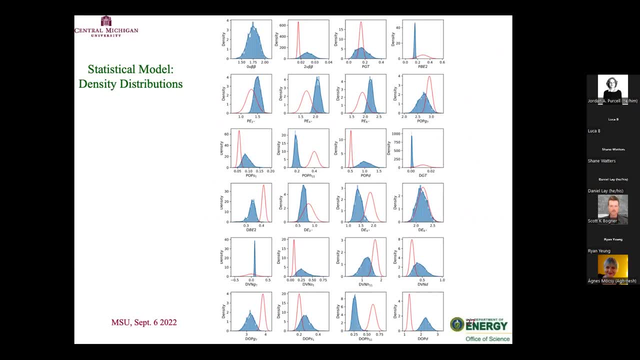 uh uh distributions. so this is what happened. and the red- what you see in red is actually a gaussian which describe the data and the uncertainty. so you see how they are compared. so in some cases are good, in some cases are not very good, like this one here, for example. the red is the data. 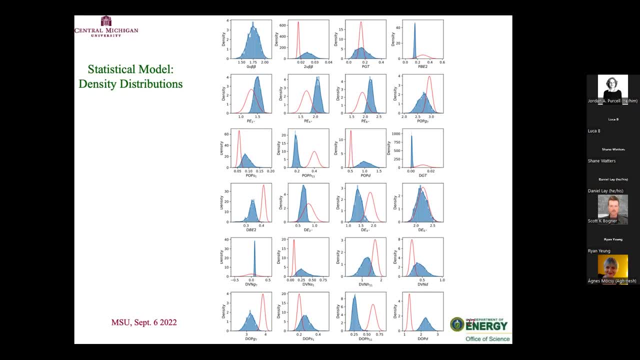 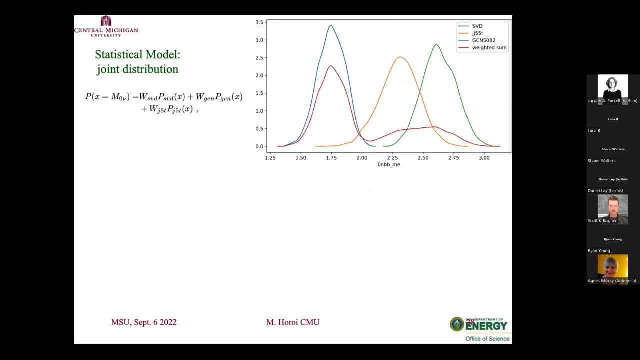 so the blue are the distribution. when i put a thousand samples- and this is this actually is for svd, is 120 one of them, right, uh, they're similar. the other they differ a little bit. but okay, so this is what it is and now let's see if we can do anything about that. so here is probably. 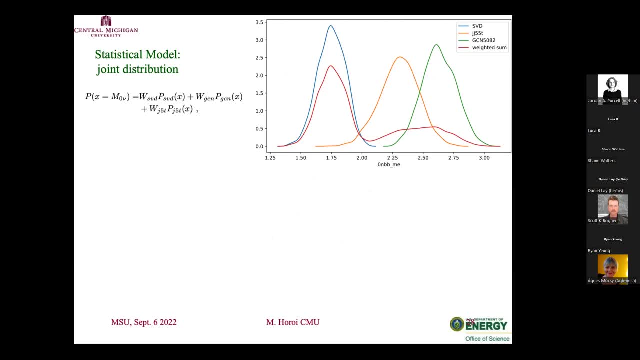 what you are interested in. so that's the main result which we can make sense a little bit of that. so i'm going to say: well, each curve with each color will correspond to a starting hamiltonian. uh, if we add the sample so you can see there are kind of. 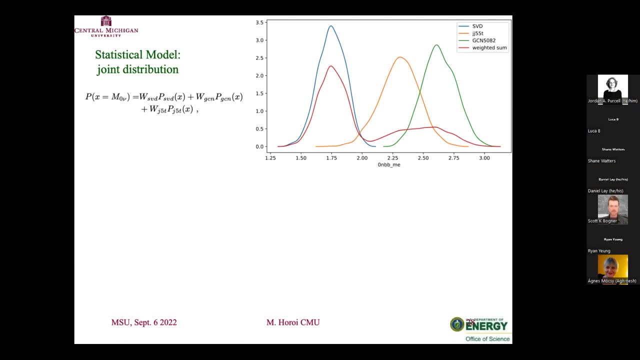 clusters, in other words they're not dispersed in many humps or anything like that. so it's quite stable to this small 10 changes random changes, right, and they are. they have different. uh, this is the blue, is svd, the middle is the jj55t, the one which i did with alex and gcn is the green. 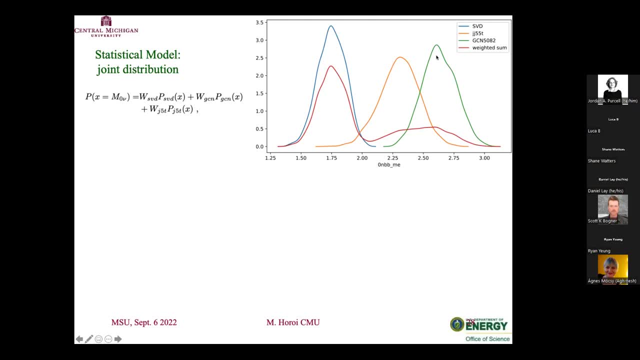 one. they see are kind of separated. they give you different, uh different average matrix elements. this is for the neutrino less matrix element and in principle we can try to do this by using the kd for each of them multiplied by some weights. the w are some weights and this weights should be extracted based on the data. it should be surmised. 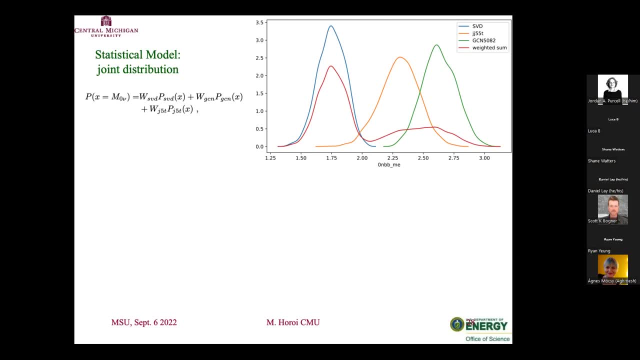 based on the data. right, as i told at the beginning, i can put w for svd one and there is zero, and now nothing gonna change. so i'm using still a bayesian point of view here, uh, and try to figure out. so for that, in order to find out, uh, how to say something about the weight. so we start with the weight and 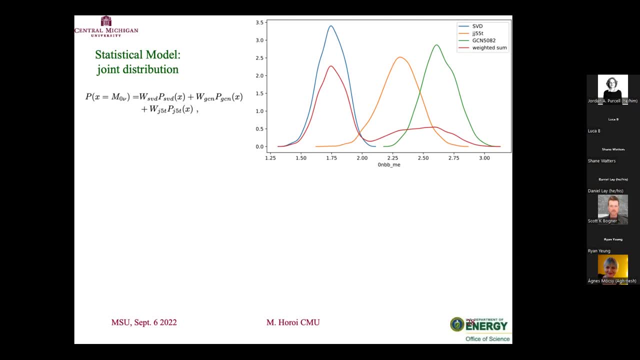 we still be subjective. remember we are subjective. so now we try to make some progress based on data. so for that we're going to use this uh statistical model called bayesian model averaging. uh, you can find it out in this uh wild, and now for a long time- and i recently, i believe people 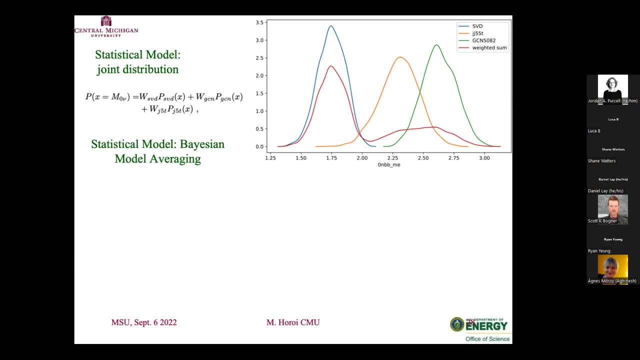 here. the vtec in particular, i believe, is very interested. i probably should also do something like that. um, so we try to figure out what are these ways based on that and the domain. the main assumption in the bayesian average model is to find out the total. 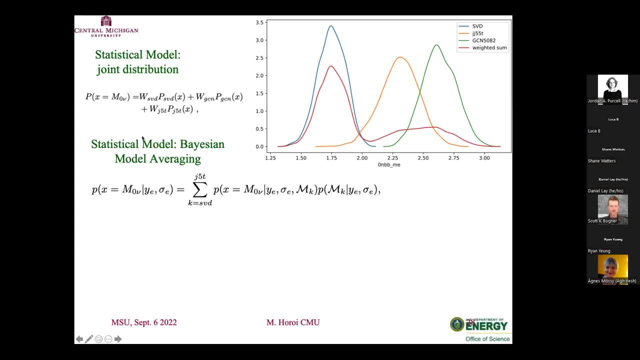 density, which in this case will be my red curve. i'm going to explain how i find that out from the three blue, orange and green. i use different weights and if i have the right weights based on information i get from the data. so data for me here will be the y and the sigma. 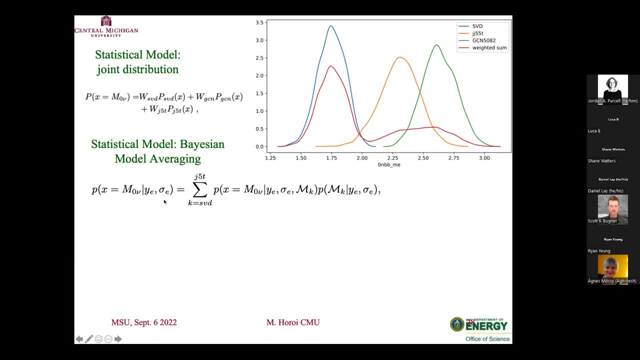 the y will be the measured data and the sigma will be their uncertainty. and the y will be the data and the sigma will be the data. so if i have the right weights, based on that, i'm going to use my statistical model to make some inference about the weights and the weights. 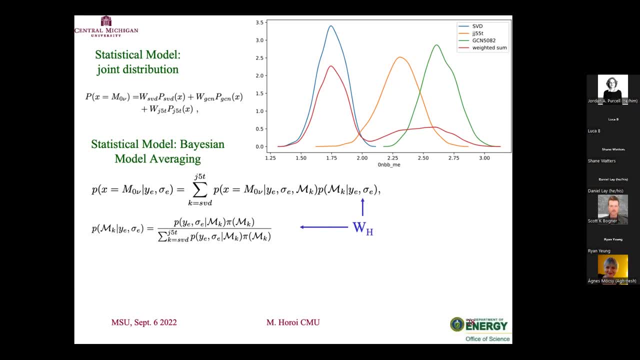 actually will be these guys. all right. so these are the weights and for the weights there is a bayesian form of calculating the posterior probability. so the weight will be a posterior based on the prior. the prior will be the pi and the posterior will be here and it will be based on the data. 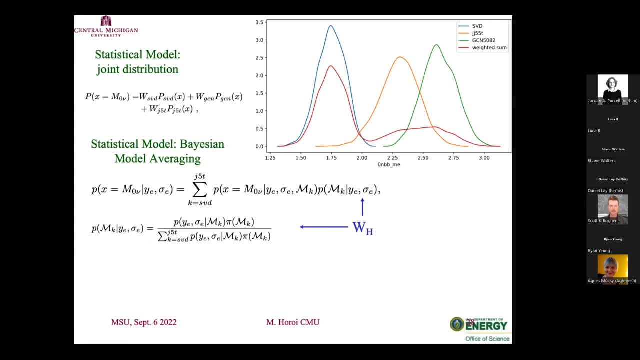 so we have. so the only thing you have to calculate this so-called evidence integral. so the evidence integrals are the stuff coming here and coming also the denominator. we're going to take the pi to be democratic. we're going to pay the prior to be one third instead of any. 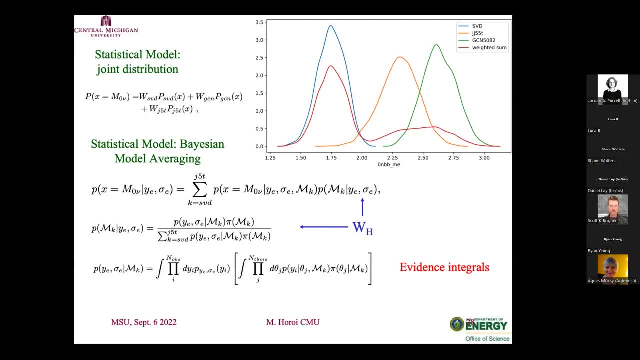 one, zero, zero, democratic- and see if we can make any progress. right, and this integral. we did so, although, okay, you may claim, okay, we have only a thousand sample. actually we calculated five thousand. I didn't do it at the analysis, but okay, remember there are 327. 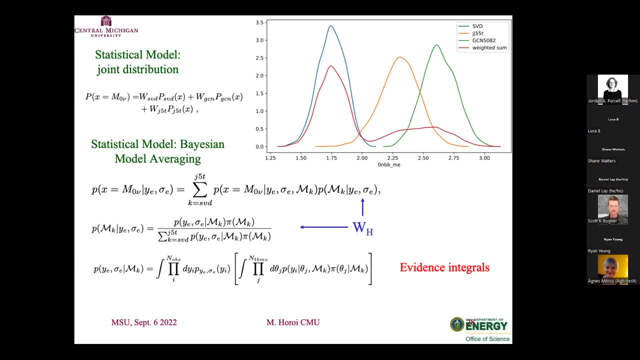 variable to integrate on. okay, so because you have, you have to do some integral on the on the two body matrix elements. here what I say is randomly sample, right, this, the two body matrix elements are randomly sample within 10% from the starting Hamiltonian. this can be done. 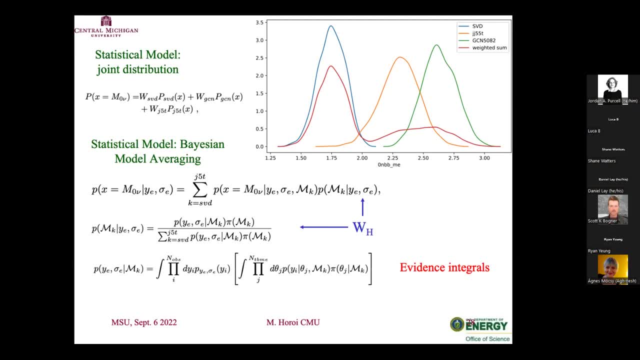 for each of them, because you can do it for each of the variables. that's, that's a beautiful part here. you have to do your own analysis for your own model. I don't have to do it for you. so the only thing is to give me this W, so in other words, the 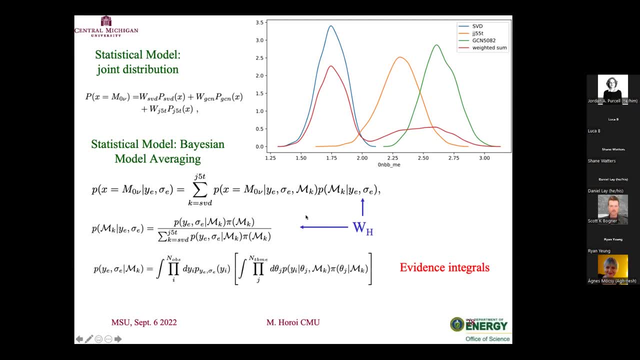 formula are going to be here. how do you how to do that? the integrals? you can do it on our own model. you have qrpa, you can do it. you have the immediate srg. if you can change some parameters, fine, okay, so this is just providing some guidance. 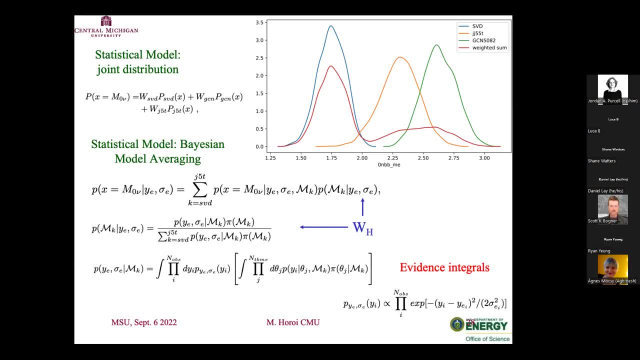 okay, so now the problem is the following: so remember, we depend on this effective charges, effective factor. turns out that if I use the number I gave to you, all right, the SVD dominates and actually everything is quite sensible to the quenching factor, the gamma of Taylor. 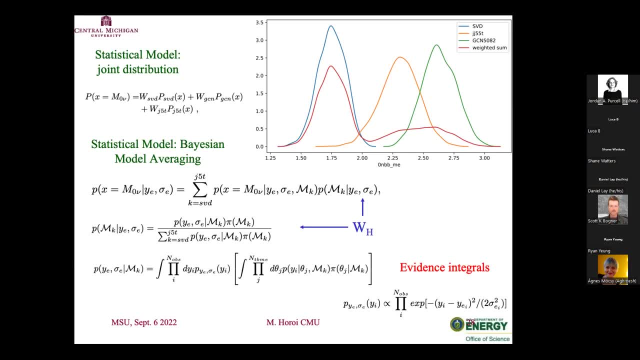 quenching factor. so if I use a quenching factor, 0.7 is just suggested by most experiments for the high end, so you're gonna get the SVD is dominated. if I go to 0.55, the JJ5T dominates, and if I get below, 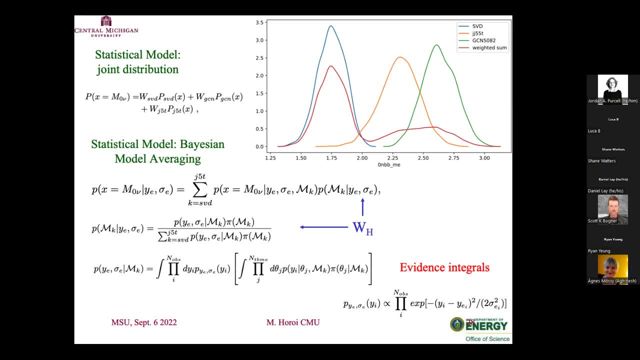 0.45, the GCN will dominate. so what do we do in this case? well, we decided to do to do Bayesian to the end, and namely, we're gonna do something in the spirit of predictor corrector, so we're gonna do an average. so we did an average between the prior 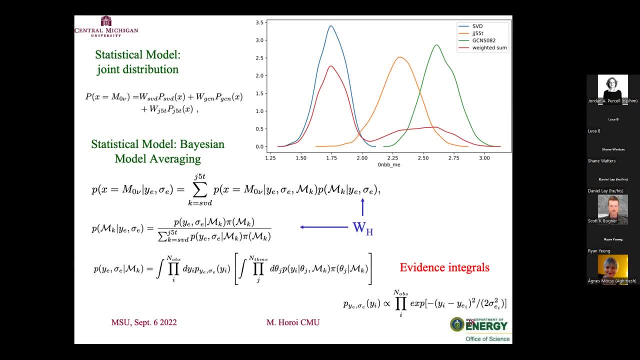 and the posterior. so in other words, the posterior come out as being one for the SVD and 0 for the other. but we did the average and that's how the the red curve coming came about okay. so I believe we are. I'm close to to the end. I have a lot. 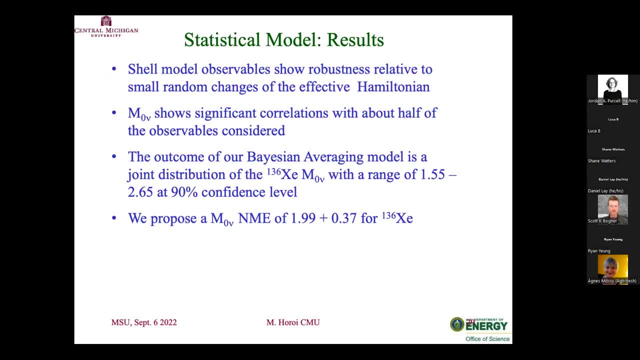 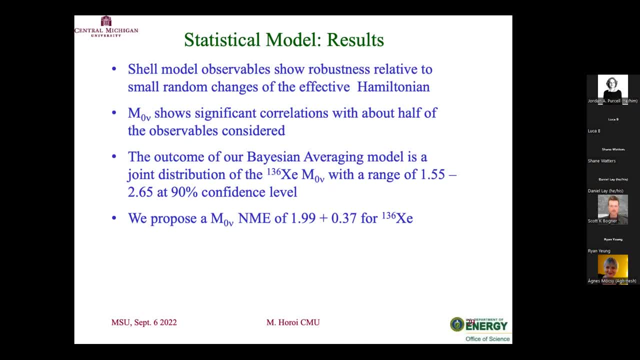 the HVD and the HVD, and the HVD and the HVD. so the new talents matrix, dimensional significant correlation was what half of your cerebral consider, let me say, repeating: they are two neutrino, they are the two plus four plus and six plus energy in the daughter and some of 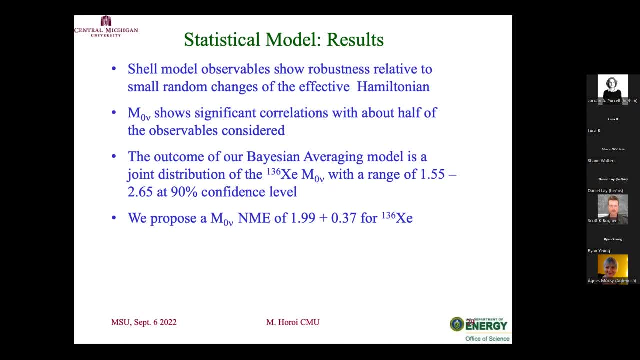 the occupation in value and vacancy for proton unit. so again. so the outcome of the base on the averaging model is a joint distribution, the one you see here being red, and, And the range at 90% confidence level is 155 to 265.. And the average is 199 plus 0.37. 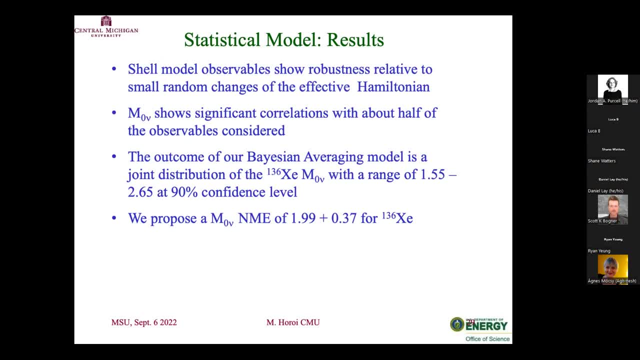 And so that's how the result. Okay, I believe. with that I'm gonna stop here. We're gonna entertain any questions. Okay, any questions local here. Sorry, I have to get back to you because I still don't understand what you did. 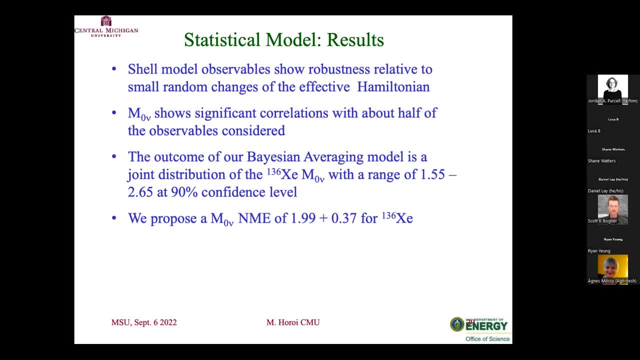 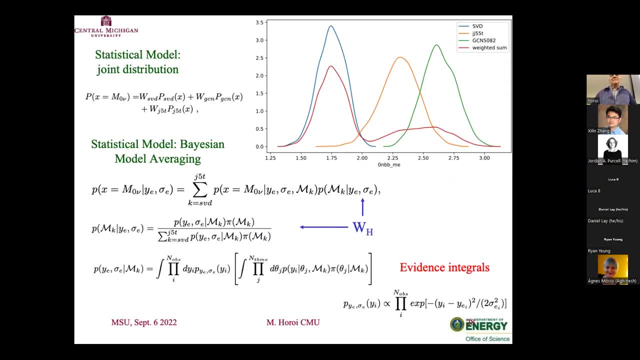 So when you start out with the and then you vary in order to generate Yeah, Or to generate The blue line, for example. So this is a blue line, is for one Hamiltonian right. So good, The two-body okay. 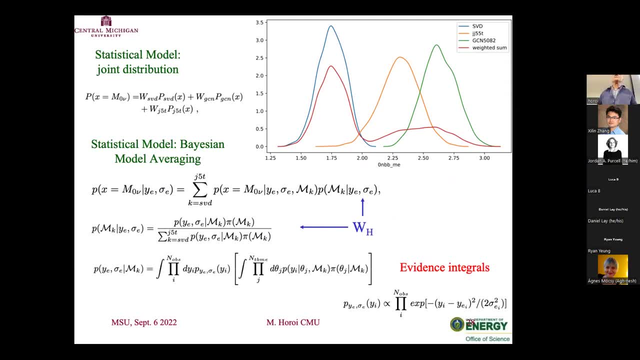 So the two-body matrix elements. So there is a shell model, Hamiltonian. After all this procedure I briefly described, it comes out with the set of two-body matrix elements And in this case there are 327 nuclear matrix elements which describe your Hamiltonian. 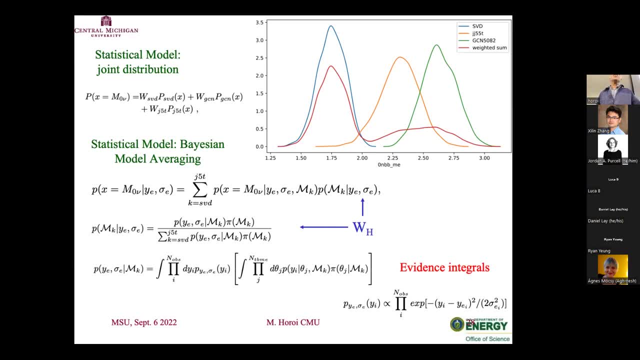 In addition to single-part matrix elements, you have single-part energy. I didn't state that I didn't want to change because this semi-magic nucleus. we decided not to change the single-part energies. So the shell model Hamiltonian has a collection. 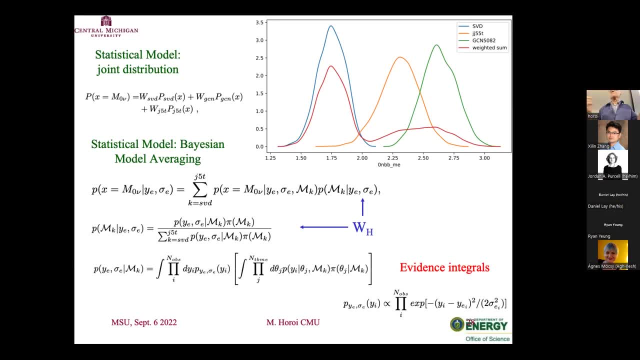 of two-body matrix element and single-part energy. So it's a one-body term and a two-body term. You said, you add and you Right randomly each of them, Each of them, yes, When you say a matrix element. 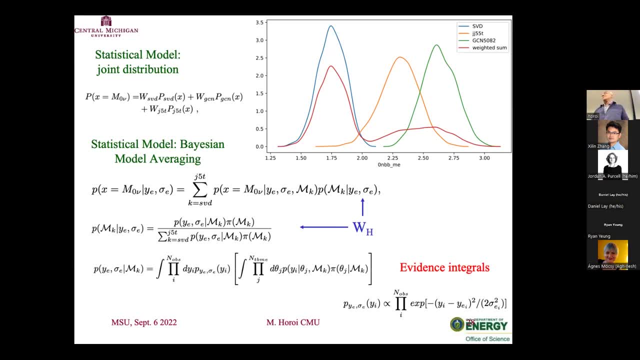 is it just a transition matrix element? No, no, Because you're not changing the energy. No, You're not changing the energy. You have a second quantization, Hamiltonian, But then I changed the energy. So you say you changed the energy. 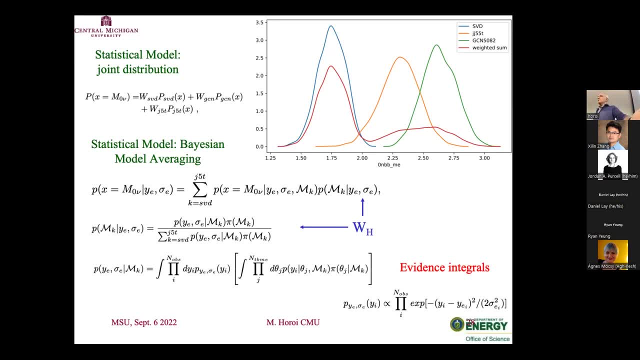 Right, So you don't change the energy. Yes, Well, yeah, but you could see that because I put the 2,, 4, and 6 there, right, You can see how they changed. OK, Then you just said a minute ago you didn't change. 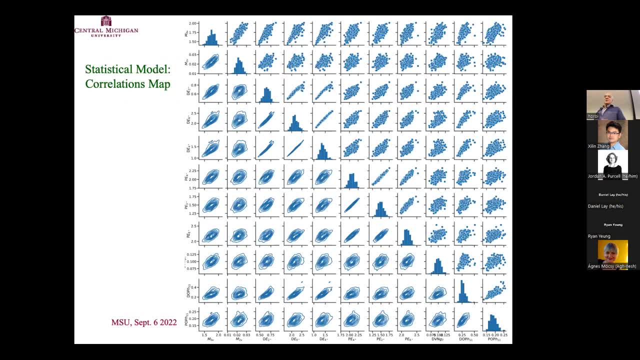 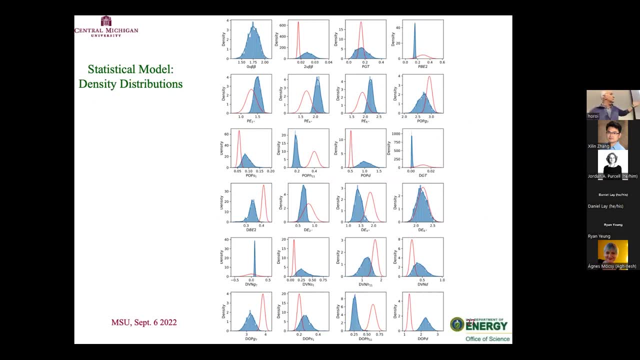 But again, I took 10% precisely because of the experience I have with, say, USDB right, So you can see this is the distribution and this is the data. right, The data is here Right Now. OK, because you come to here you may say: why do you see this Gaussian for the E2?? 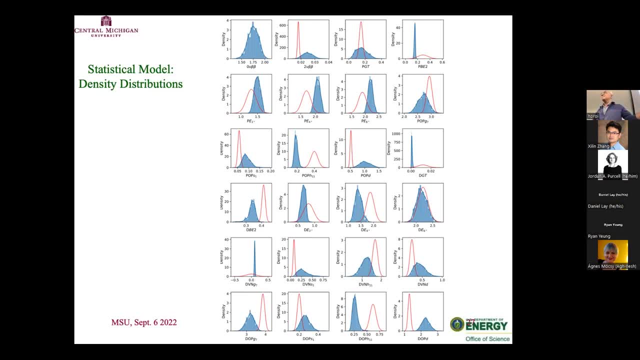 It's because the energies they have, basically they are almost exact, right, So they have KeV. It depends on your detector. You measure gamma rays for that. But again, I put the error. you see, here is actually the error I can calculate. 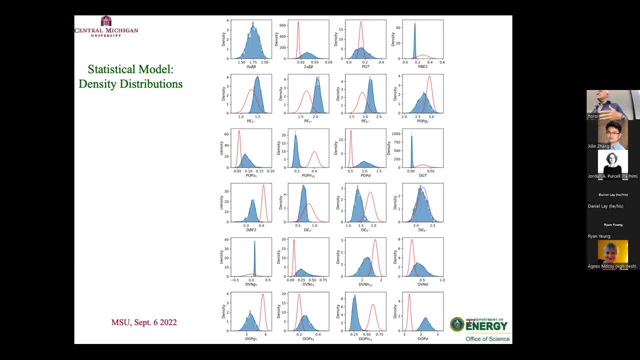 Each of the Hamiltonians, Each of the Hamiltonians have an RMS. The RMS is a deviation from the experimental energies. So I use for that the RMS for that. So for the red curve, red curve for the energies. that's what it is. 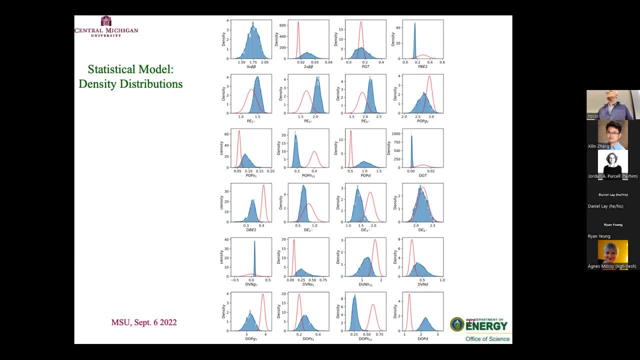 The principle is a line at the center, but that's what it is, OK. so, yes, I have not finished my question. OK, because you started it. So you said that the R and E2 get back to the same protocol. 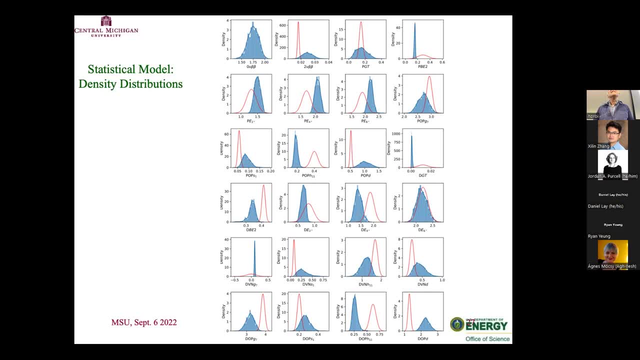 That you have a mutual. So initially, these Hamiltonians are generated with some certain protocol. Yeah, that's, that's, that's. You know exactly. Do you see the fact, or is it whatever? No, we just let me say again: 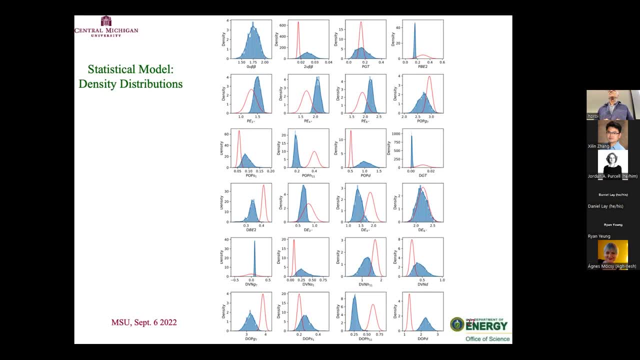 We just vary the effective Hamiltonian. You vary the effective Hamiltonian, You are using the same. And now the most important question is: what are you prior on these major cellulose? So are you varying? Well, I'm, I'm not, I'm not OK, but again I'm not here. 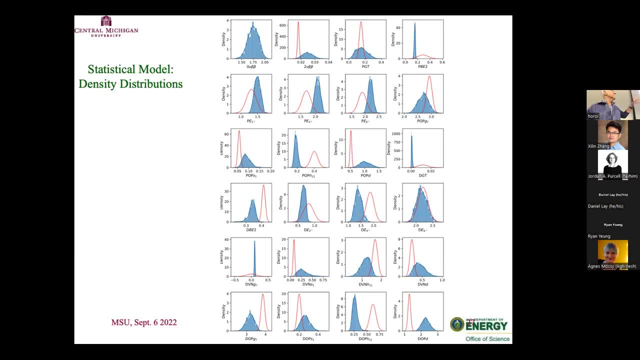 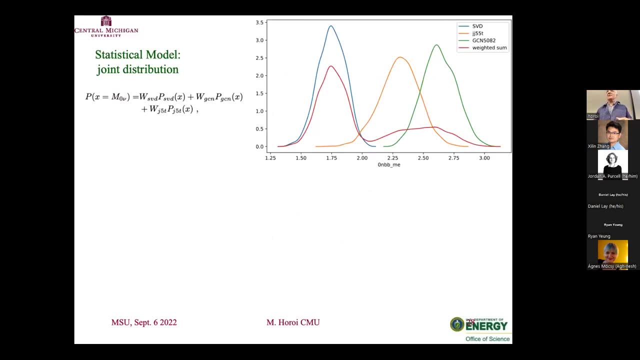 I'm not making a statistical analysis of the Hamiltonians, but of the neutrino less though better decay matrix element. So my priors for that are one cell, one cell, one cell for each of the three Hamiltonian. I don't have priors for my head. 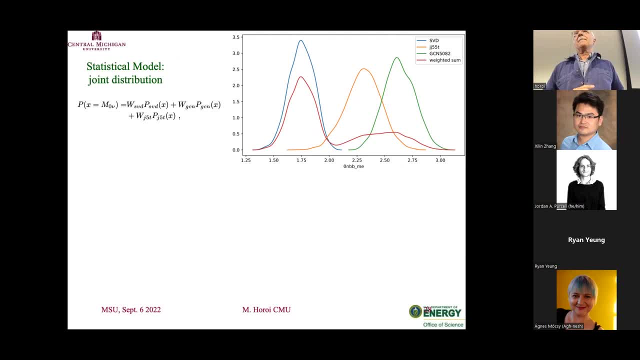 Yeah, From some Distribution. Yeah, What is that Distribution? As I told you, it's uniform. No, but how good. 10%. Oh, I missed that, Sorry. Oh, so you're, you're, you're. 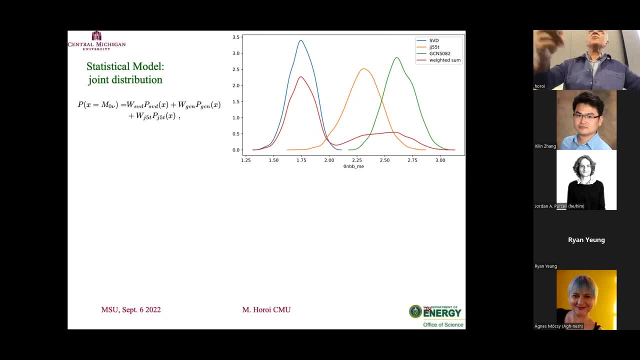 I wanted to say. then I explained why 10%. now we did 50, we were going to do 15%, but 10% is based on the experience between the USDA and the SDB. So USDA is giving you good energies without changing too much the original matrix elements, because I'm worried that if I do that, I change. 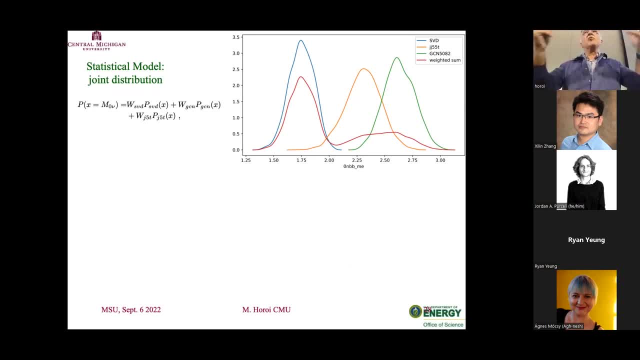 The phases in the way function they're going to not give me. because I only fine tune energies, I'm going to get the wrong observables and apparently that that's the case. So, based on that, I decided for 10%. Okay. 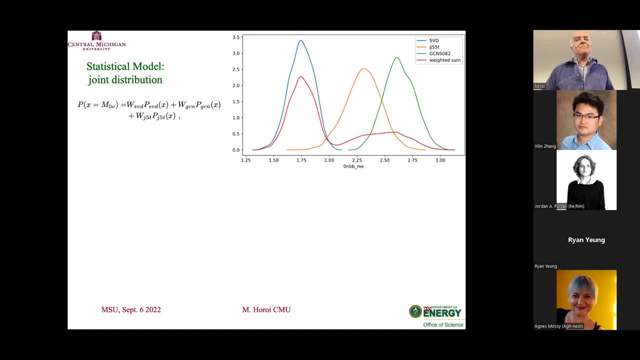 Go ahead. Let me ask you a simple question: Um GA, the function and the effect of charges. Um, why didn't you just use a statistical prior on that? Now, Right, That could be an extension. I mean, if you want to split here a little more. 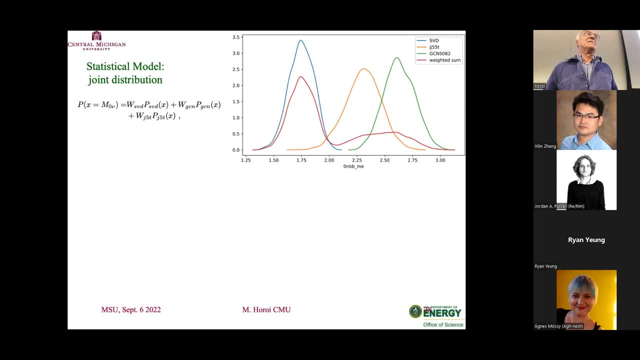 Yeah, sure. So so the last part, where you talked about the value of the fighting that you would assume, how it led to this effect of waiting, this Bayesian, everything is based on here, So so maybe you could, Let's find that again. 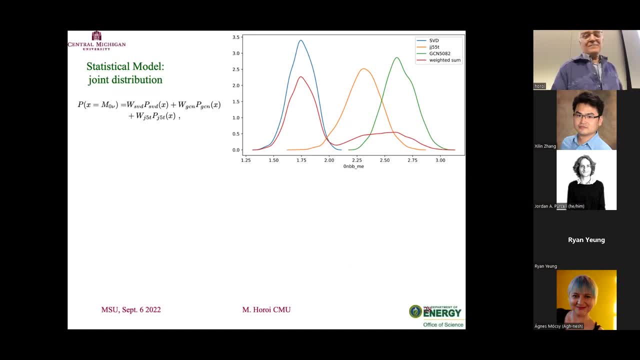 The shows you explored different values of GA, and that- Not GA, not GA. I disagree on your GA. I disagree on that. GA is 1.27.. So what we have here is just quenching of the matrix element. It's not. it's my belief and many others. 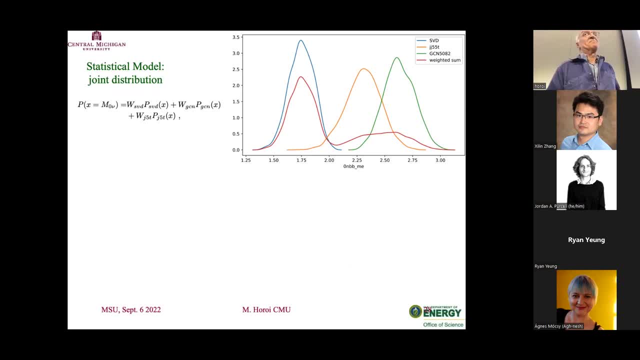 So I'm going to disagree with you. The GA is quenched. Oh, okay, No, no, I, I. I just mean the quenching factor for yeah, Okay, So again. so for most of the cases people study, they use quenching factor of around 0.7 for every nuclear light. 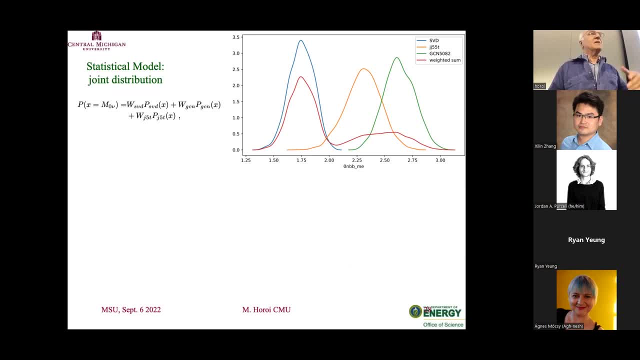 We're going to people are going to tell you the piece. We're going to give you 0.9, but the FBA, FBA and uh uh, JJ for four up to 100, give you good Number. 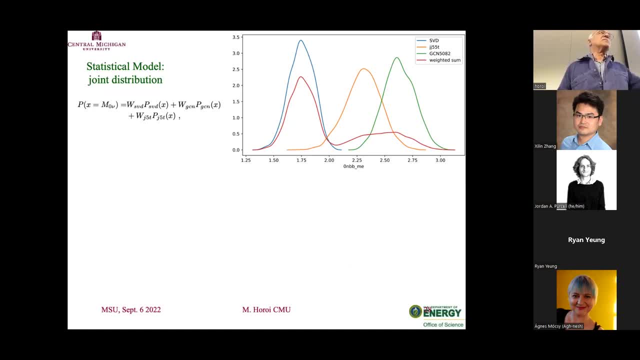 So we always calculate the two neutrino matrix element with 0.77.. If I use a Hamiltonian, which is not too much changed in that case works fine, So that the advantage of the blue curve here, because this one is only T, equal one matrix element. or what change in teen isotopes to get a good, effective Hamiltonian. 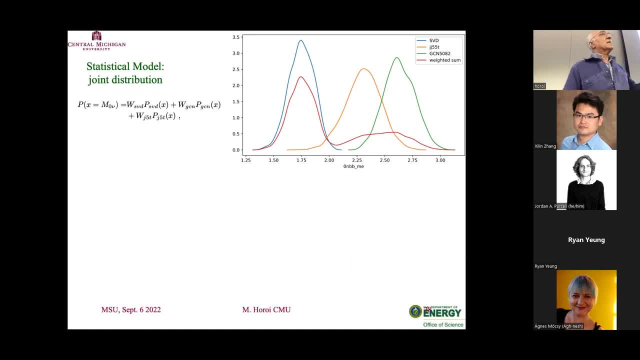 They don't get as good energy as GCN, but on the other hand it preserved the original matrix Selma And so you don't need to amend. So people which are using the GCN Hamiltonian they they want to describe the two neutrino matrix element. 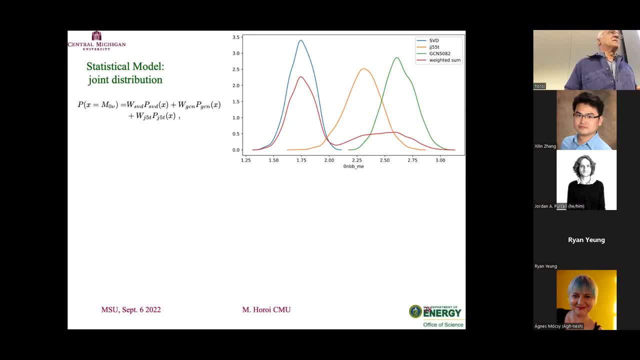 They did a quenching of 0.35, meaning that there'll be a factor of four in the observable. So that's what's my point, if you want. So I made my choice. This is Bayesian, but I made my choice, boys. 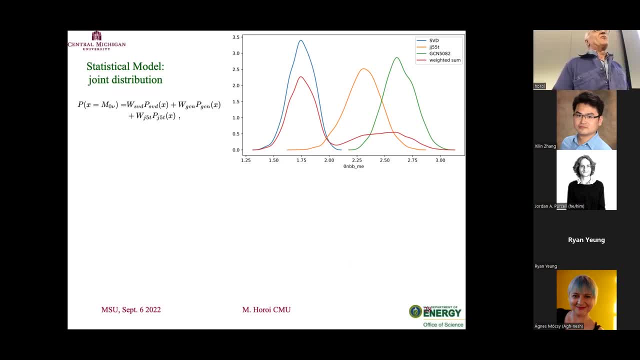 I'm going to use 0.7 for everything, for everyone And, as I say, we are curious. In that case, give me the prior, the posterior, give me one for blue and zero for the others. But I make an average here because I'm still a Bayesian. 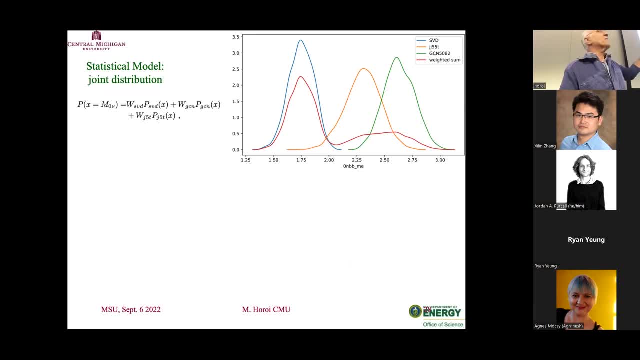 If I change the quenching factor, if I go from 0.7 to 0.55, now the curve in the middle give you dominates, And if you go down to 0.45, you're going to start getting the green curve dominant. 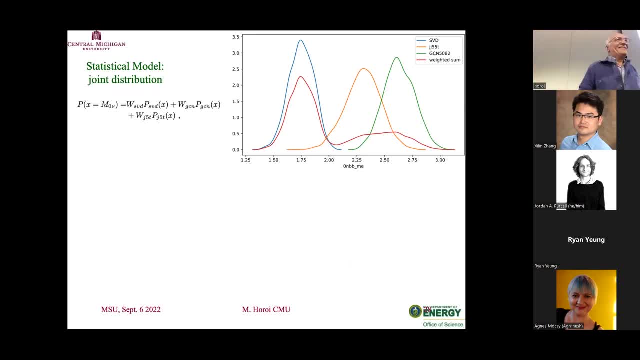 But we are Bayesian, So this is our belief. So that's the whole point here. Do they have a Harvard method? I'm still puzzled here. So your prejudice is around 0.7.. Yeah, that's my prejudice, So that's a prior. 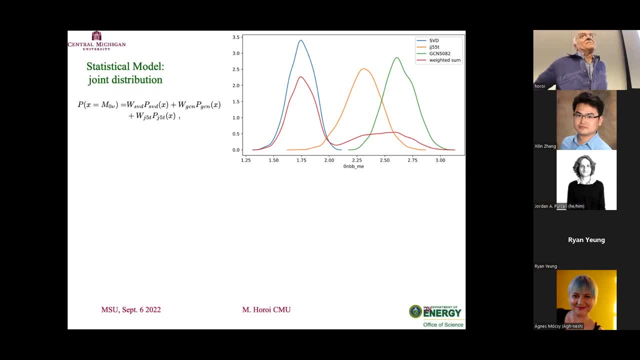 And that affects the weight of your three moments. More general questions. These are three. The model is the same. It's the same model- space, And so what about limitations of the shell model? Yeah, So what about the limitations? So there are a lot of limitations, in particular, 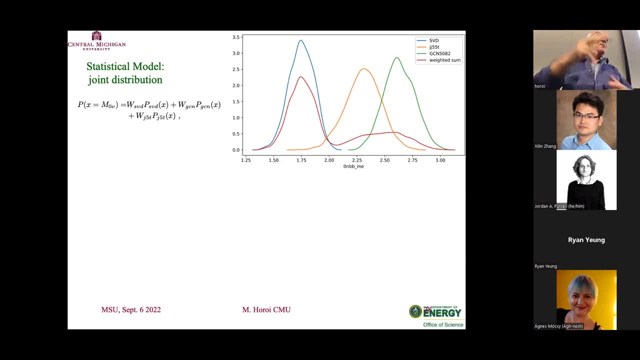 I mean, first of all, they capture the most salient feature, The feature of the nuclear structure, because it describes all the level of Fermi surface And for relatively low energies that's probably most of it right. So there are people who are making a claim that, okay, you should use larger model spaces. 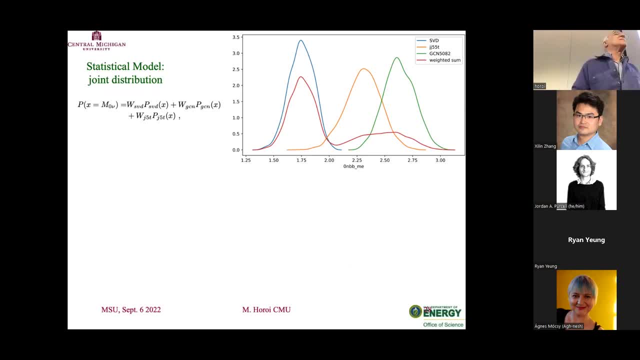 Or at least to you know, get effective. Hamiltonians, which are a little more precise, like Heiko is doing, They start from a big model space And after that they Reduce consistently to a smaller model space, But in principle, in the end they use the same model space. 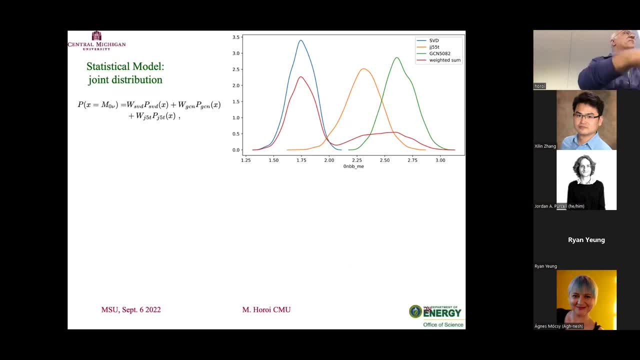 Only they're effective Hamiltonian and they have an effective operators which encapsulate a little bit of the physics beyond your model space. Okay, Now I didn't say that I go quickly, So the question would be: do you have any effective operator? 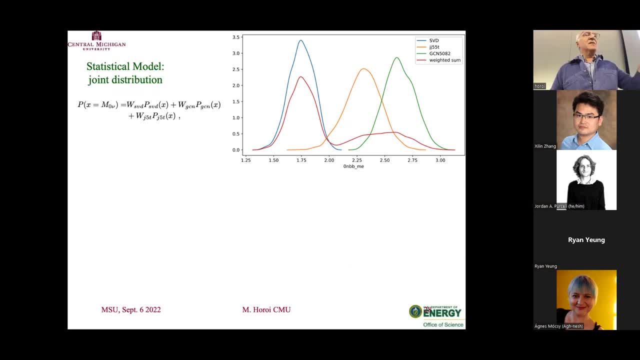 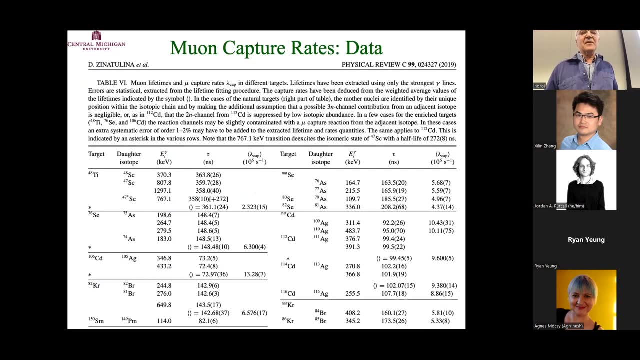 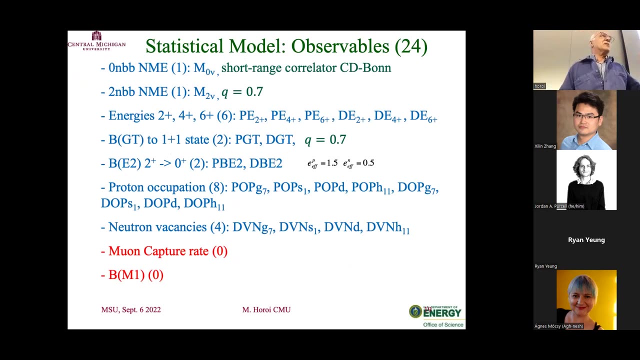 And my answer is yes, And on the list- I'm not sure if I can go quickly back, Maybe I can. On the list- is the fact that the effective piece here is this: here, The shore range correlator. So this is going to quench your matrix element. 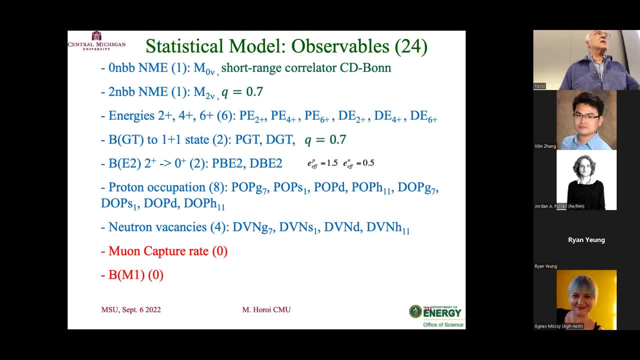 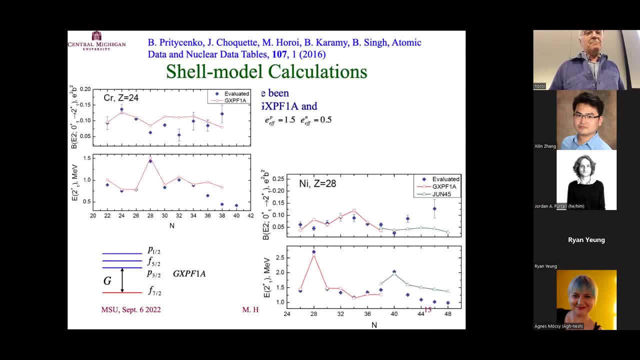 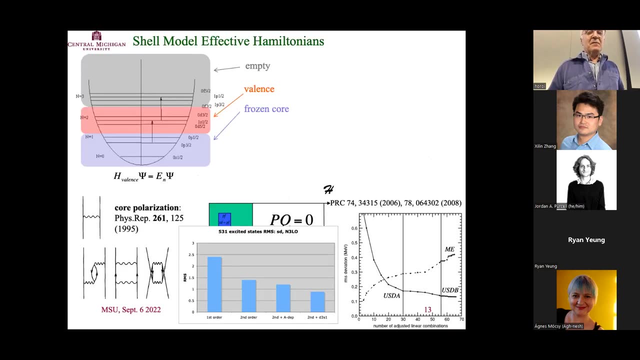 It's not a quenching factor, It's a quenching operator which describes, gives you some effectiveness about your shore range things. So probably, if you can see here I have, When I wrote the matrix element, I put some dots because I'm sure that some of the reviewers there are some dots. 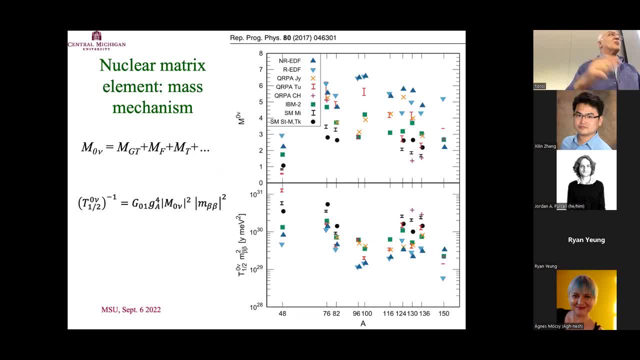 Some people are calculating right now something called a contact factor. This is more specific to kind of perturbation theory. So in other words, you have to have a consistent description of the shore range correlation for your entire model space. It turns out that, for example, 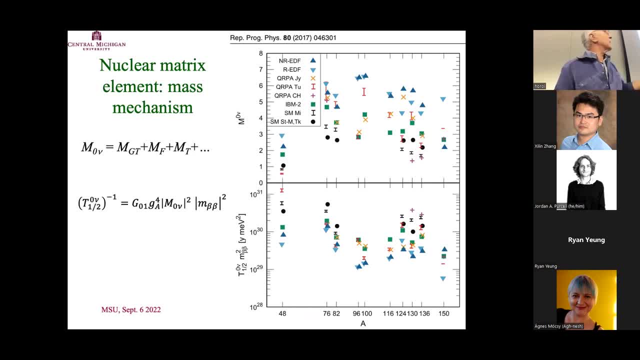 a HICO gets 0.6.. If it doesn't use the contact factor, it gets 0.87 if you use it, So in my case with my correlator, actually I get 0.85.. So I think that I am fine-tuning my effective operator, my shore range correlator, to some more ab initio calculation, not to the data. 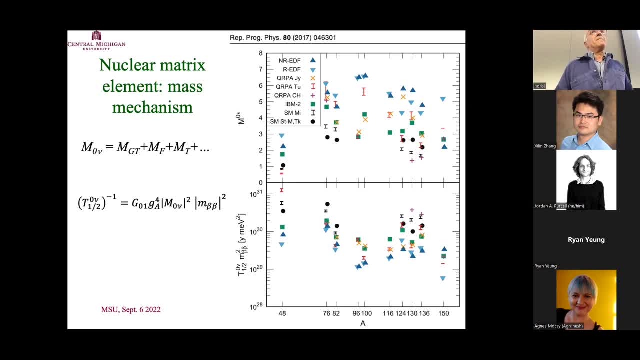 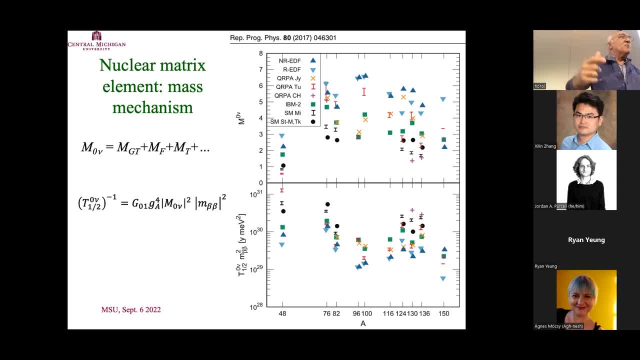 Instead of saying my prior is 1 for me and 0 for all, the other, and I let you primary is 2.. Pi of f Democratic Three shows modals with 10% confidence level over 1% confidence level over 20%. 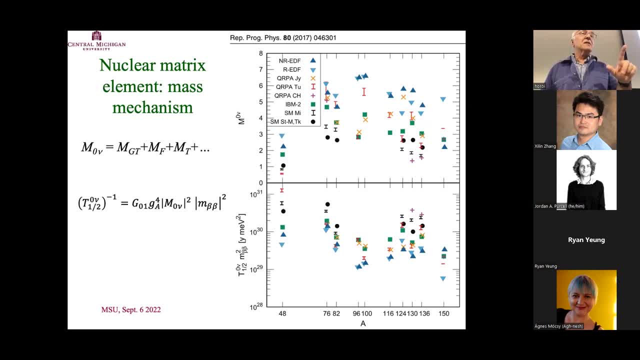 Yeah, Yeah, Let me say again: everyone can do the same thing. The challenge is to do this integral here, So everyone, they're independent. The analysis, this, this. Let me see if I can go quickly. All right, 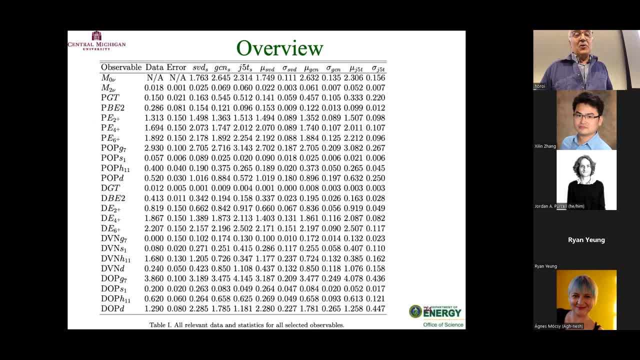 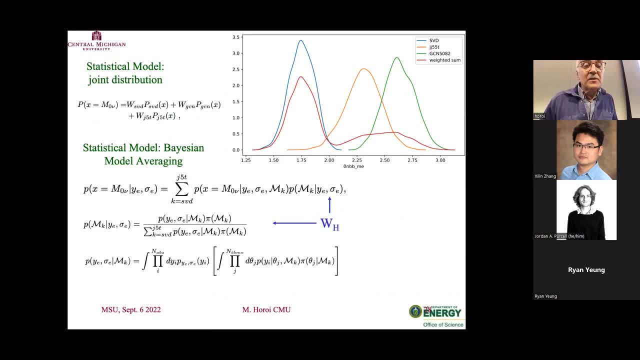 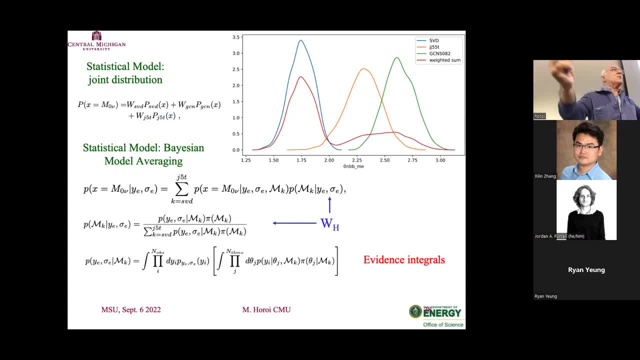 OK, OK, OK, OK, OK, OK. So every you have your own model, do your that, and if you can compare with me, that's fine. So, and the pilot, the prior, said for me one third, one third answer in this case something I'm pretty democratic. 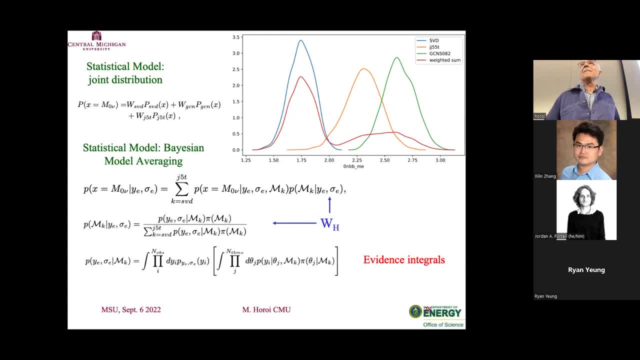 So I have. the first one is what the message? if you're in the sort of yourself and every driver getting by 10% when you chose to fly, or have your final uncertainties, I think will be twice or a half. So my community says I think will be very important to touch base data while you're doing. 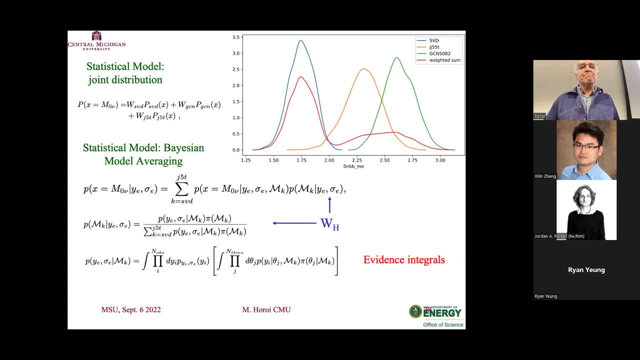 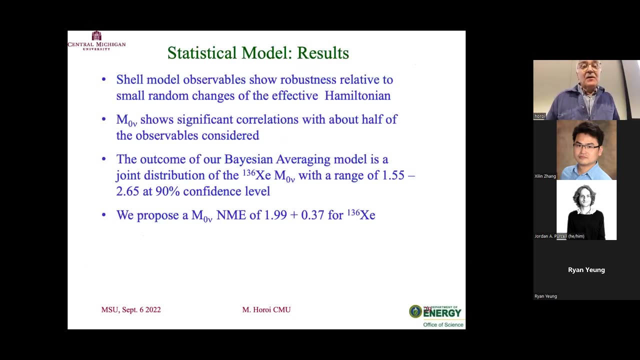 that like being or some sort of figure that will, yeah, yeah, so we can, we can, we can think about doing the, the, the, that actually the first step. okay, so probably let's see if i have it on my conclusion. uh, maybe not. oh, i'm sorry, i have some.